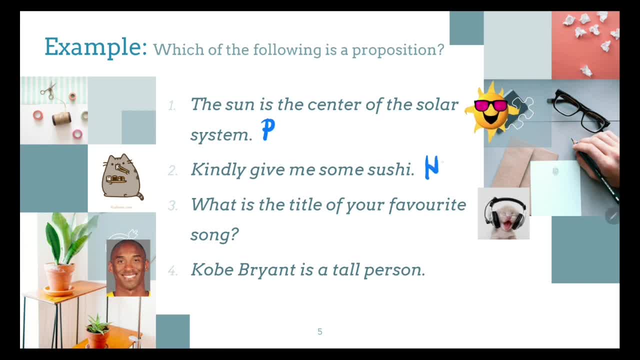 Obviously, this is not a declarative, so not a proposition. What is the title of your favorite song? It's a question, therefore, not a proposition. Kobe Bryant is a tall person. It is a declarative, but there is a question if it's true or false. 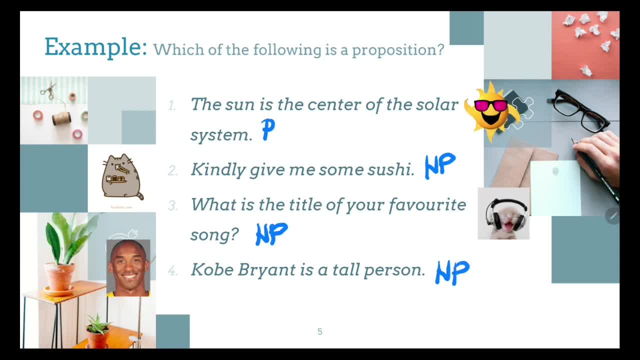 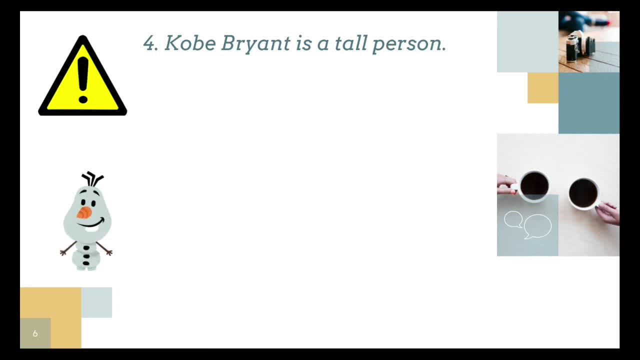 So this is not a proposition. Let's go back with the fourth. Kobe Bryant is a tall person. Why is this statement not a proposition? Yes, it is true that he is tall, but maybe for those who are shorter than him. So it is true. 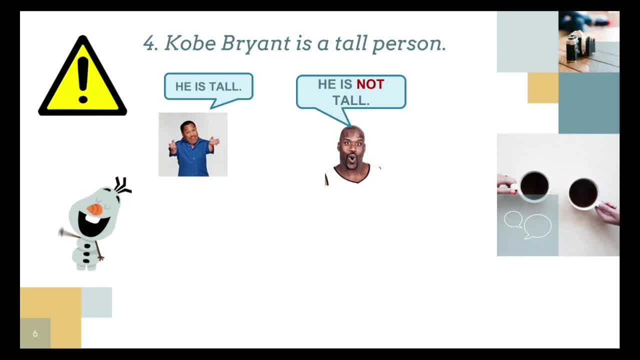 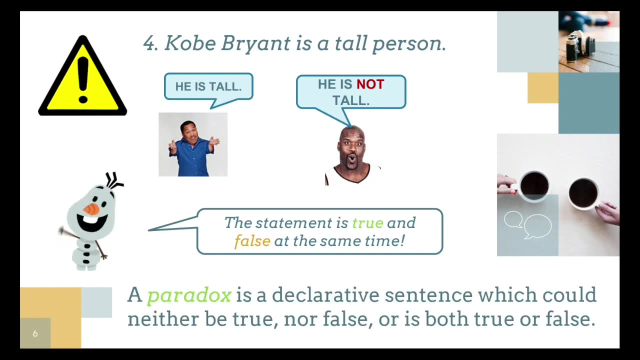 But for some who is taller than him, he is not tall. So this statement is true and false at the same time. So that makes this statement not a proposition, because it cannot be both true and false. Statements like this are what we call a paradox, a declarative sentence which could neither be true nor false, or is both true or false. 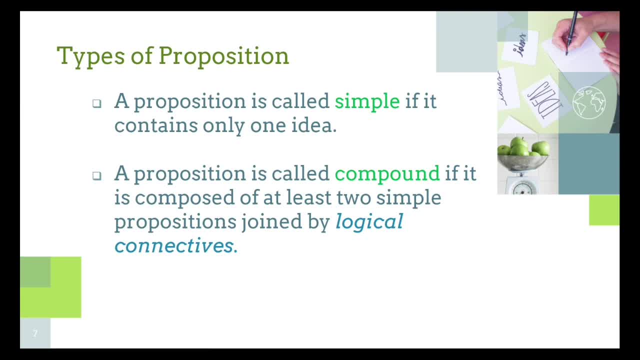 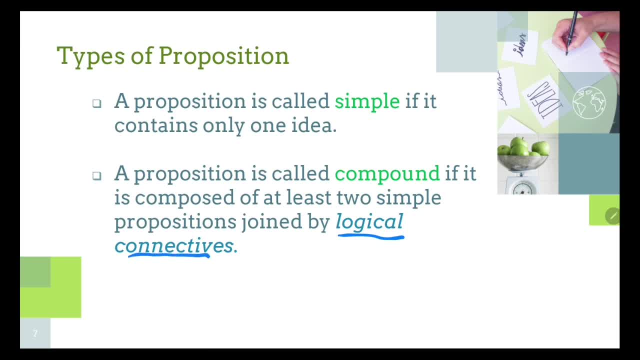 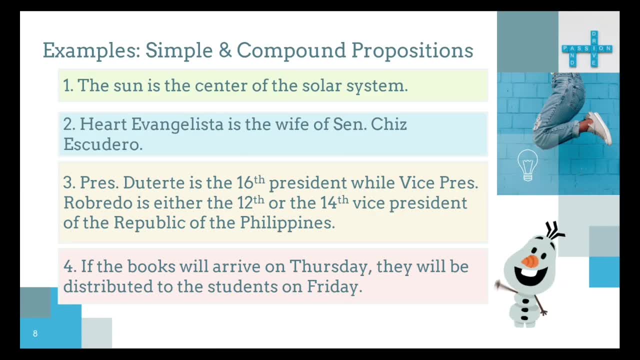 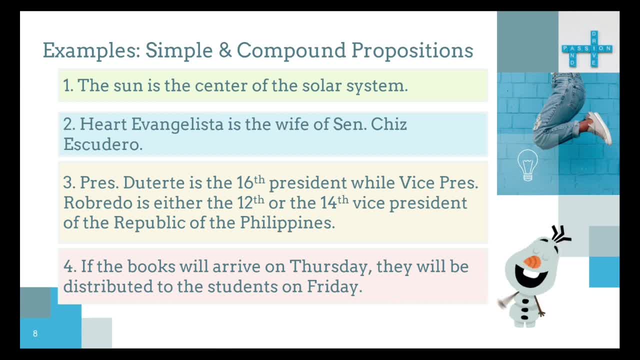 President to 30 is a 16th president, while Vice President Obrado is either the 12th or the 14th vice president of the Republic of the Philippines. If the books will arrive on Thursday, they will be distributed to the students. 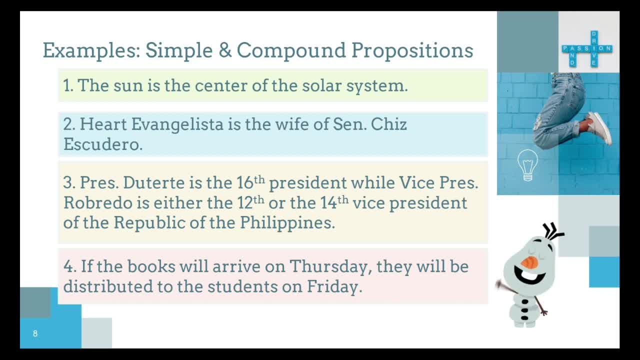 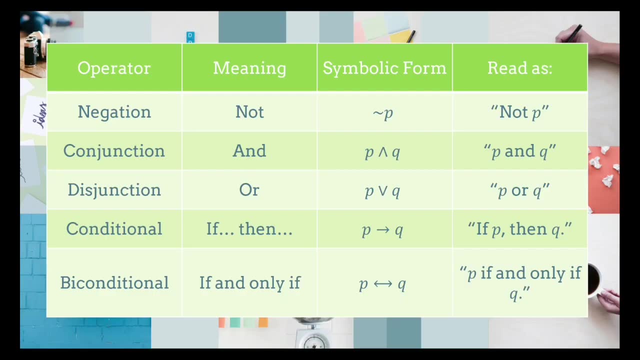 on Friday. so statements one and two are simple, while three and four are compound propositions. basic logical operators. do we have negation, conjunction, disjunction, conditional, and by conditional, along with their meaning, symbolic form and how you read them. not P, P and Q, P or Q. if P, then Q, P, if and only if Q. let's start. 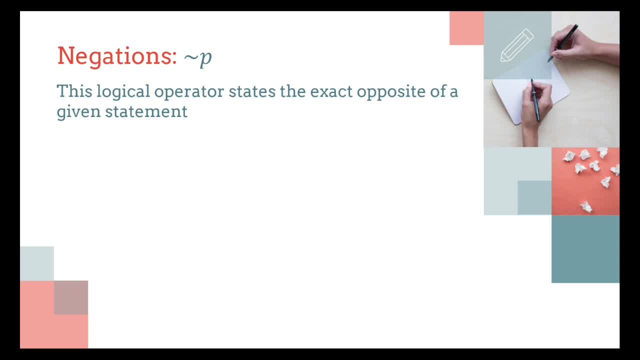 with negations. this logical operator states the exact opposite of a given statement. P. the sum of two odd numbers is even, so the negation would be: the sum of two odd numbers is not even. next Q. it is sunny today, so the not Q would be: it is not sunny today. there are only two possible. 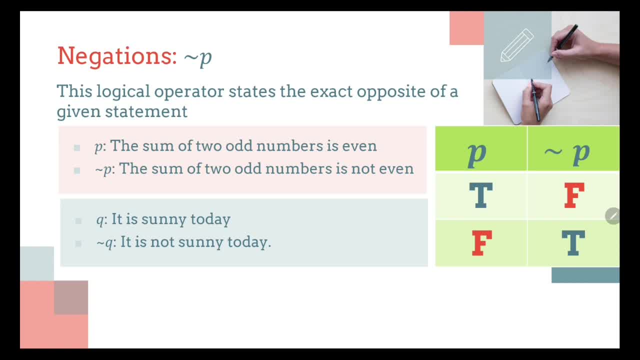 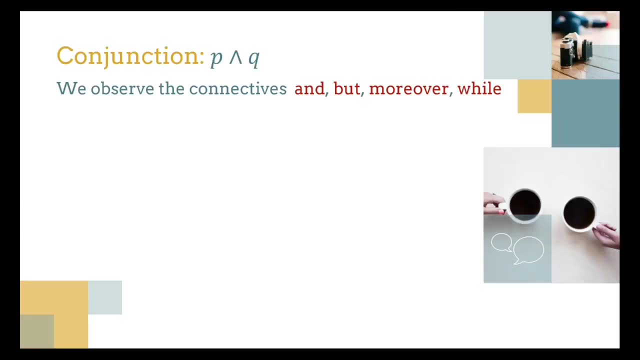 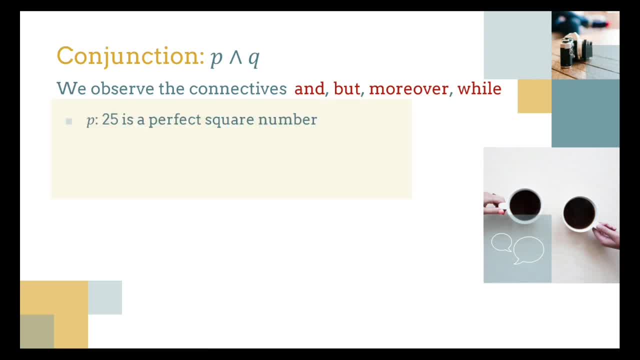 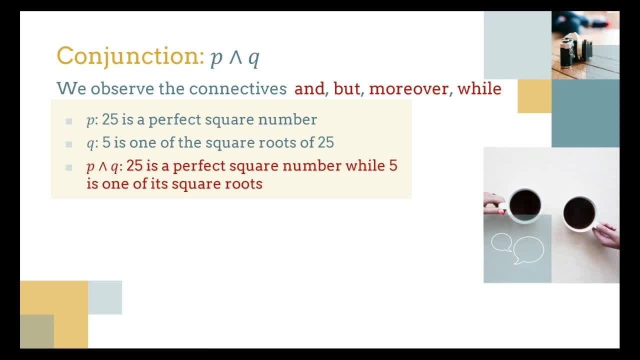 number and you have Q. 5 is one of the number and you have Q. 5 is one of the square roots of 25, then P and Q 25 is a square roots of 25, then P and Q 25 is a square roots of 25, then P and Q 25 is a perfect square number, while five is one. 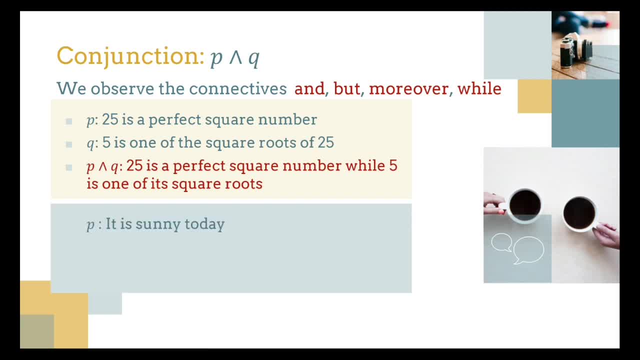 perfect square number, while five is one perfect square number. while five is one of its querets. next P, it is sunny today. of its querets. next P, it is sunny today. of its querets. next P, it is sunny today. Q I need to go to work. P and Q it is. 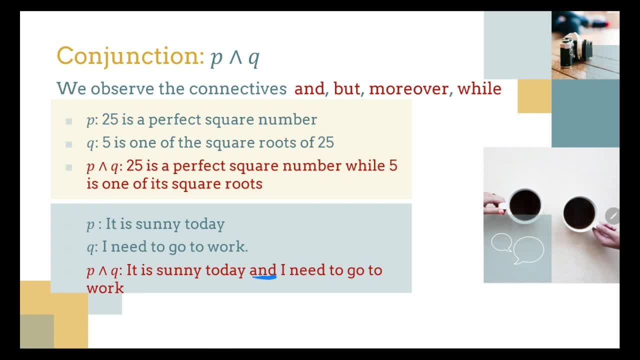 Q I need to go to work, P and Q. it is Q I need to go to work, P and Q. it is sunny today and I need to go to work. so sunny today and I need to go to work. so sunny today and I need to go to work. so we have here the truth. table of a. 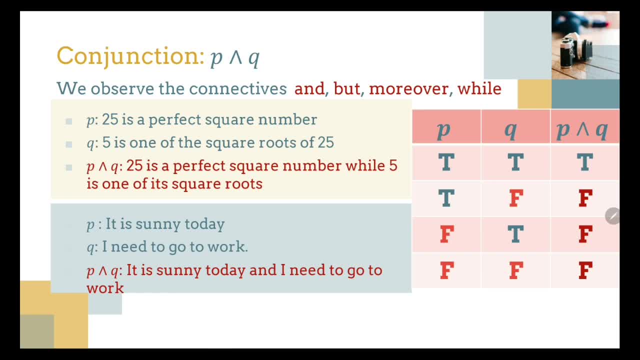 we have here the truth table of a. we have here the truth table of a conjunction. if you know this, we have conjunction. if you know this, we have conjunction. if you know this, we have four rows because we need to take all four rows, because we need to take all. 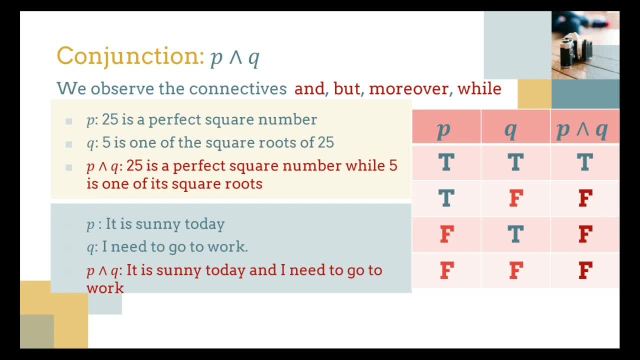 four rows, because we need to take all the possible combination of the truth. the possible combination of the truth, the possible combination of the truth. value of P and Q- both true, true. P is value of P and Q- both true, true. P is value of P and Q, both true, true. P is true and Q is false or false P and Q is. 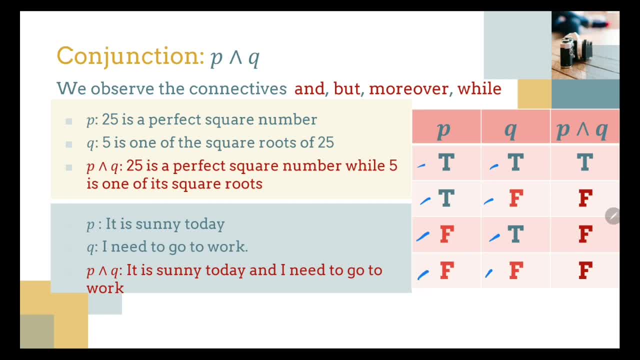 true and Q is false or false. P and Q is true and Q is false or false. P and Q is true or they're both false. so you have true or they're both false. so you have true or they're both false. so you have four possible combinations for the truth. 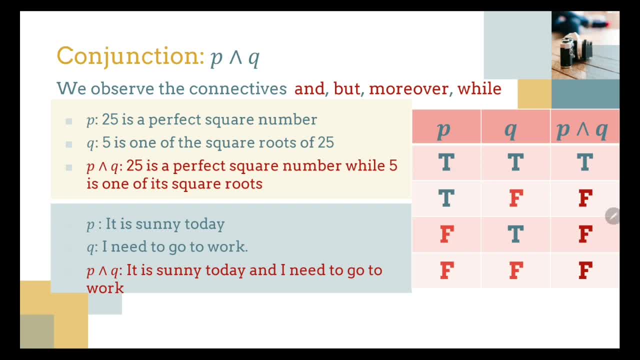 four possible combinations for the truth. four possible combinations for the truth: value of a conjunction: if both are value of a conjunction. if both are value of a conjunction. if both are true, then the conjunction is true. if true true, then the conjunction is true. if true true, then the conjunction is true. if true- false, then the conjunction is false. 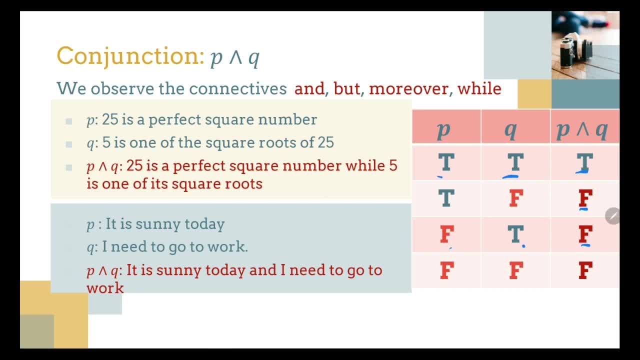 false, then the conjunction is false. false, then the conjunction is false. if false, true, then the conjunction is. if false, true, then the conjunction is. if false, true, then the conjunction is false, is false, false and the conjunction false, is false, false and the conjunction false, is false, false and the conjunction is false. if you know this, the 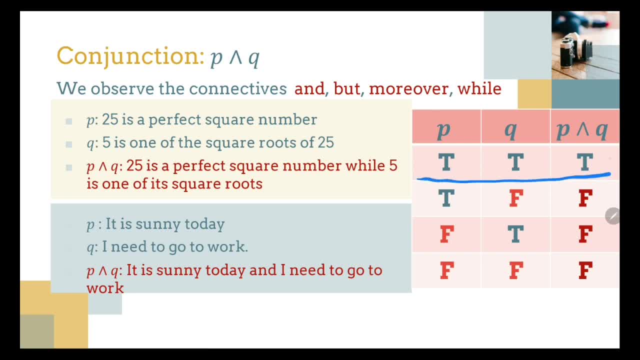 is false. if you know this, the is false. if you know this, the only time our conjunction is true, if only time our conjunction is true, if only time our conjunction is true. if they are both true, they are both true, they are both true. next disjunction: we observe the words or: 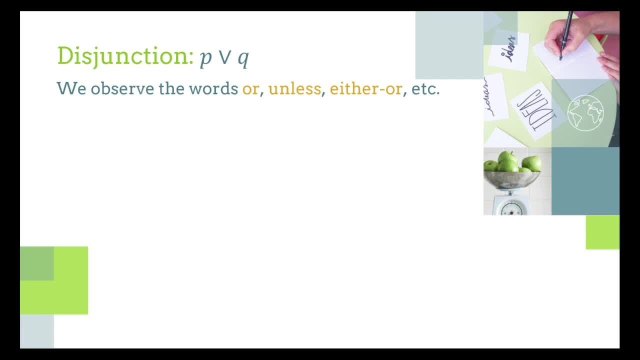 next disjunction, we observe the words: or. next disjunction, we observe the words: or unless, either or etc. or in short, or unless either or etc or in short, or unless either or etc or in short. or example: P Mary will buy her clothes at. example: P Mary will buy her clothes at: 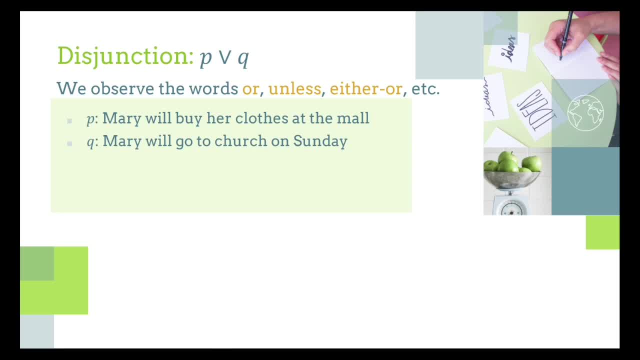 example: P Mary will buy her clothes at the mall. Q Mary will go to church on the mall. Q. Mary will go to church on the mall. Q Mary will go to church on Sunday. so P or Q either Mary will buy Sunday. so P or Q, either Mary will buy. 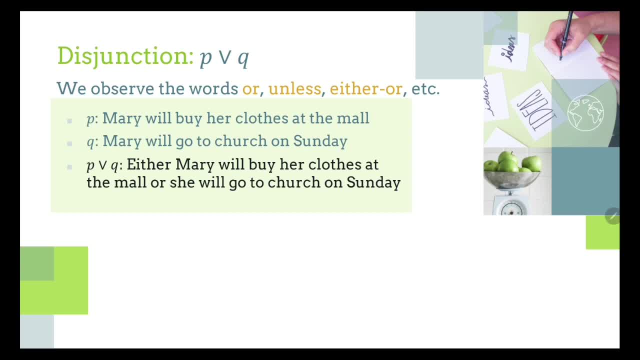 Sunday. so P or Q: either Mary will buy her clothes at the, her clothes at the, her clothes at the mall, or she will go to church on Sunday mall. or she will go to church on Sunday mall, or she will go to church on Sunday. so there is the or affair, next P it is. 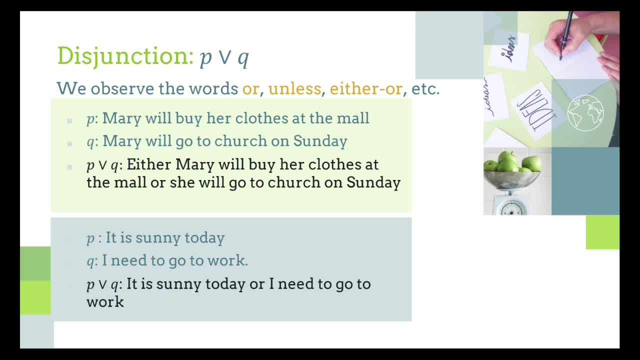 so there is the or affair next P. it is. so there is the or affair next P. it is sunny today Q I need to go to work. so sunny today Q I need to go to work. so sunny today Q I need to go to work. so it is sunny today or I need to go to. 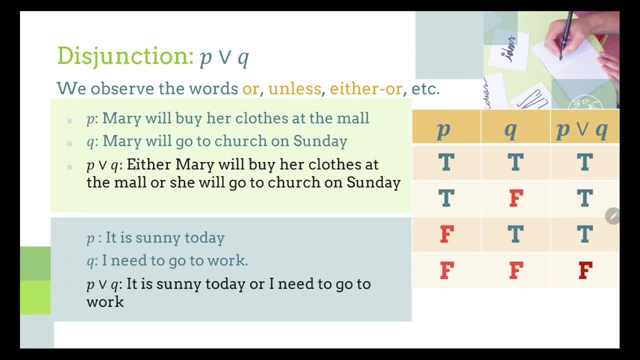 it is sunny today or I need to go to. it is sunny today or I need to go to work, and here we have the truth table work. and here we have the truth table work. and here we have the truth table for the disjunction. a same combination. 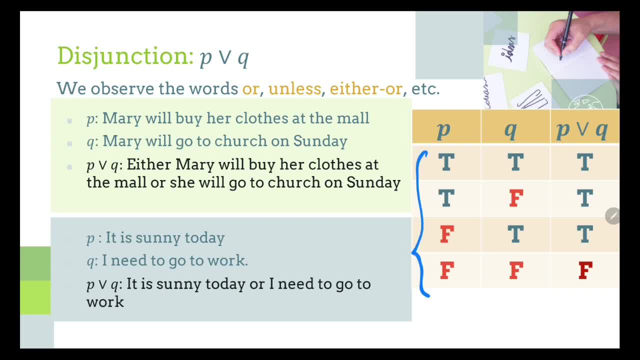 for the disjunction, a same combination for the disjunction, a same combination of the truth value of P and Q, if you, of the truth value of P and Q, if you of the truth value of P and Q, if you notice the only time the disjunction is. 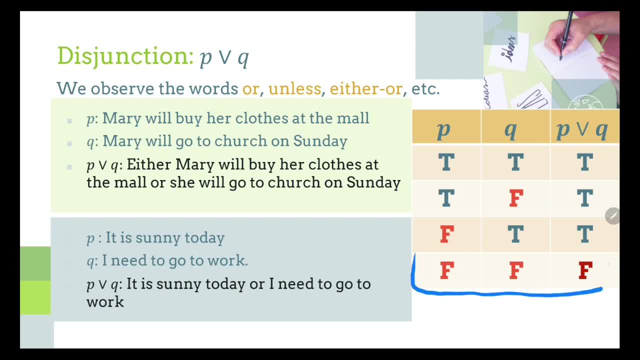 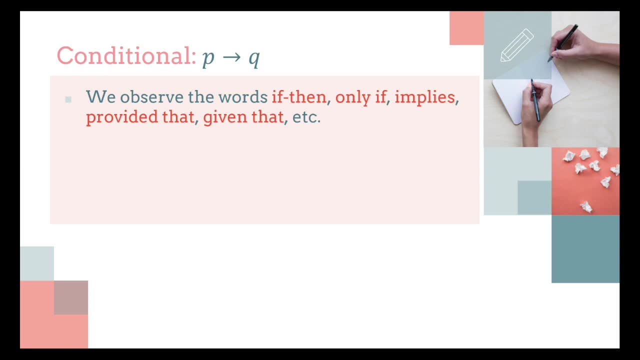 notice the only time the disjunction is: notice: the only time the disjunction is false is when both are false. so if at least one of them is true, then so, if at least one of them is true, then so if at least one of them is true, then the disjunction is true. conditional: we: 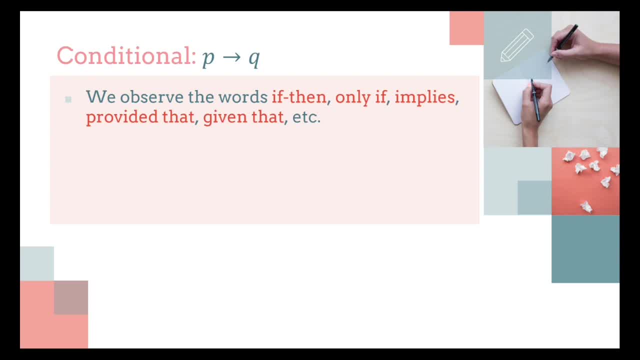 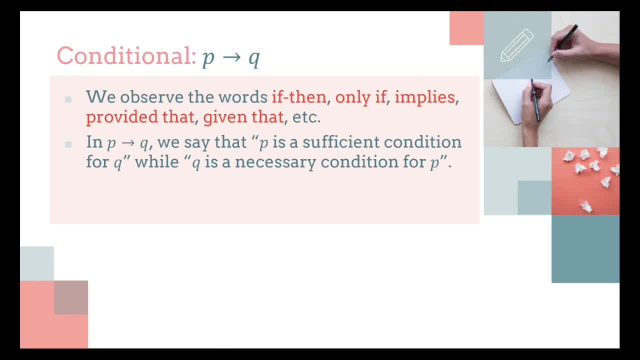 or implies, provided that, given that, etc. in a conditional statement we see that, etc. in a conditional statement, we see that, etc. in a conditional statement we see that P is a sufficient condition for Q, P is a sufficient condition for Q, P is a sufficient condition for Q, while Q is a necessary condition for P. P is. 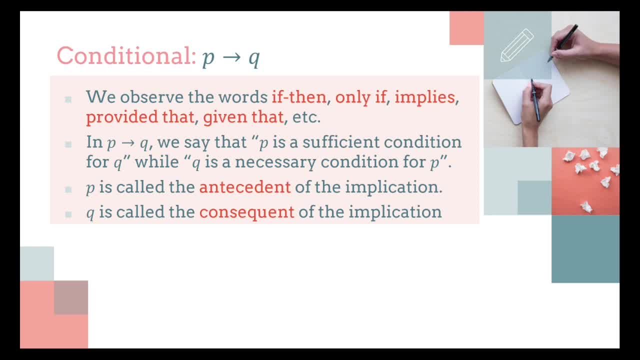 while Q is a necessary condition for P, P is. while Q is a necessary condition for P, P is called the antecedent of the, called the antecedent of the, called the antecedent of the implication, and Q is called the implication and Q is called the. 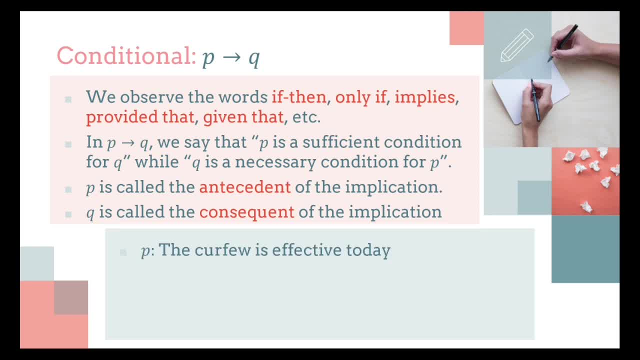 implication and Q is called the consequent of the implication example. consequent of the implication example. consequent of the implication. example: the curfew is effective today and the? the curfew is effective today and the? the curfew is effective today and the Q is the police officers will arrest. 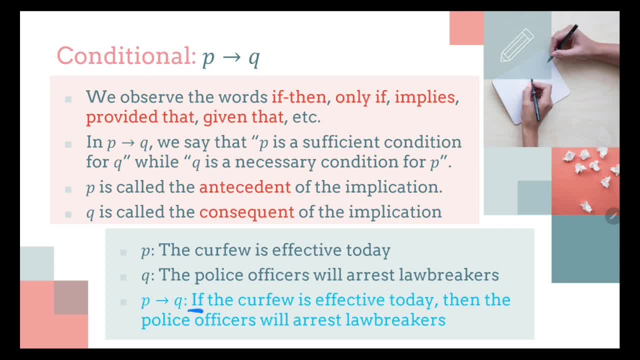 Q is the police officers will arrest. Q is the police officers will arrest lawbreakers, if the curfew is effective, lawbreakers. if the curfew is effective lawbreakers. if the curfew is effective today, then the police officers will. today, then the police officers will. 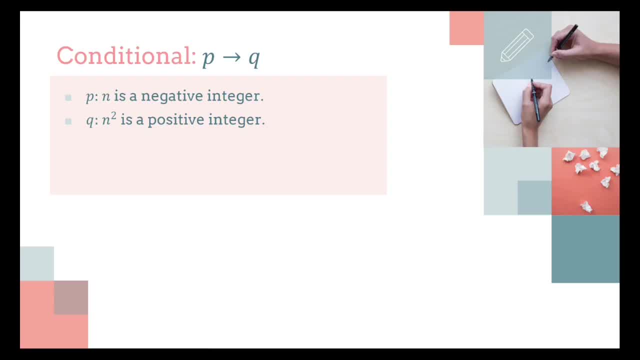 today, then the police officers will arrest lawbreakers. another example: P? n arrest lawbreakers. another example: P n arrest lawbreakers. another example: P? n is a negative integer. Q n squared is a is a negative integer. Q n squared is a is a negative integer. Q n squared is a positive integer if n is a negative. 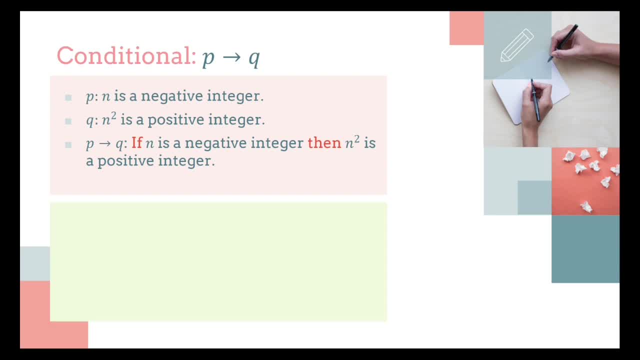 positive integer if n is a negative positive integer. if n is a negative integer, then n? squared is a positive integer, then n? squared is a positive integer, then n? squared is a positive integer in an implication. it means that integer in an implication. it means that integer in an implication. it means that if P is true, then Q is also true. 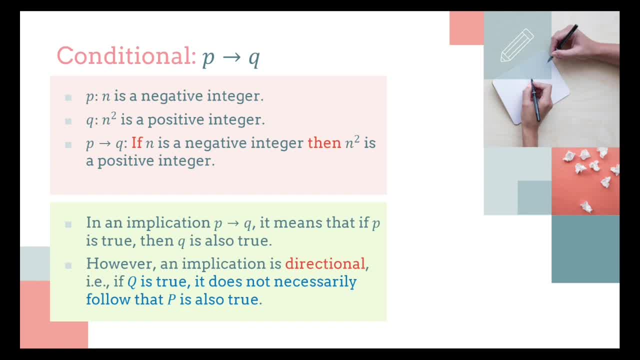 if P is true, then Q is also true. if P is true, then Q is also true. however, an implication is directional. however, an implication is directional. however, an implication is directional. example: if Q is true, it does not example. if Q is true, it does not example. if Q is true, it does not necessarily follow that P is also true. 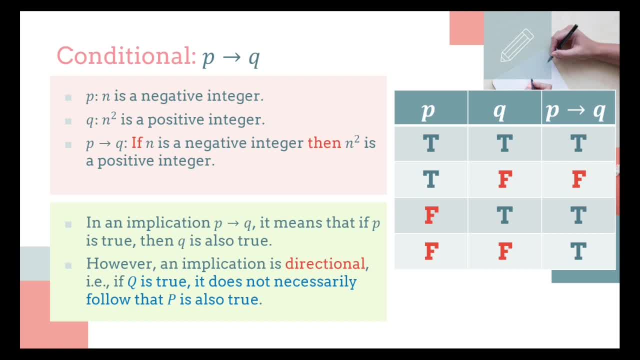 necessarily follow that P is also true. necessarily follow that P is also true. let's look at the truth table of a. let's look at the truth table of a. let's look at the truth table of a condition, if they are both true, true condition. if they are both true, true. 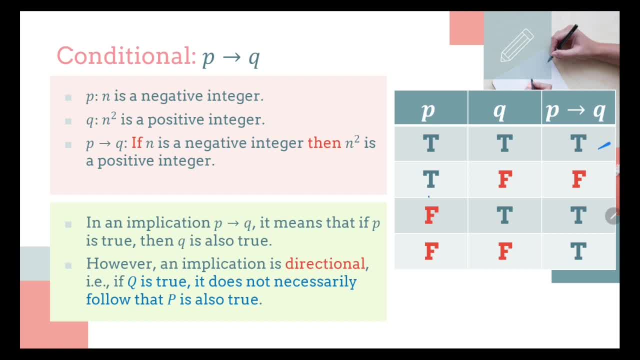 condition. if they are both true, true, then it is true. if P is true and Q is, then it is true. if P is true and Q is, then it is true. if P is true and Q is false, it is false. why this is false? it is false. why this is? 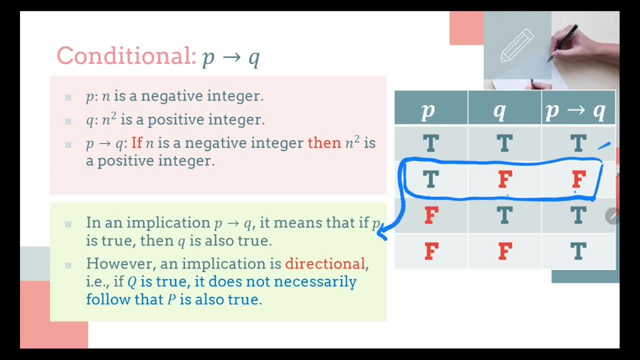 false. it is false. why this is false because of this. it means that if P is false because of this, it means that if P is false because of this, it means that if P is true, Q must be true. that's why the true Q must be true. that's why the 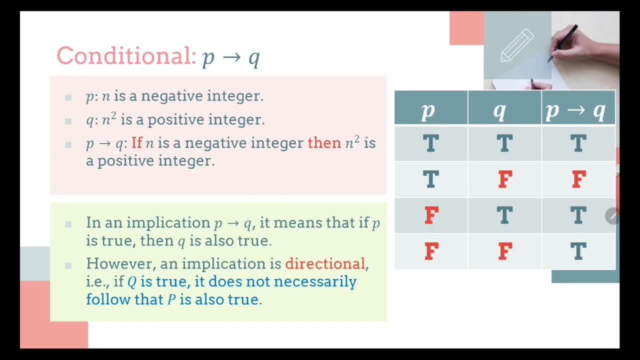 true, Q must be true. that's why the condition I is false. the third one: if P condition I is false. the third one: if P condition I is false. the third one: if P is false in Q is true, it is true because is false in Q is true, it is true because. 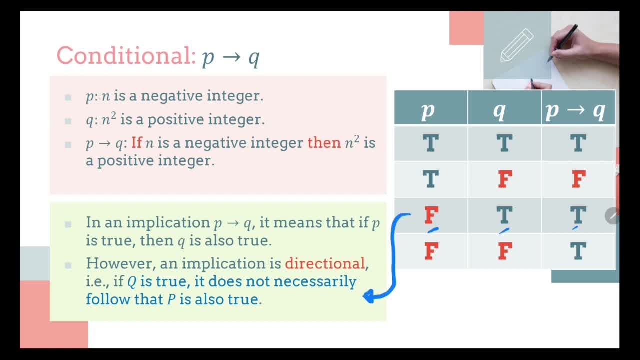 is false in Q is true. it is true because of this. that if Q is true, it does not of this. that if Q is true, it does not of this. that if Q is true, it does not necessarily follow that P is also true, necessarily follow that P is also true. 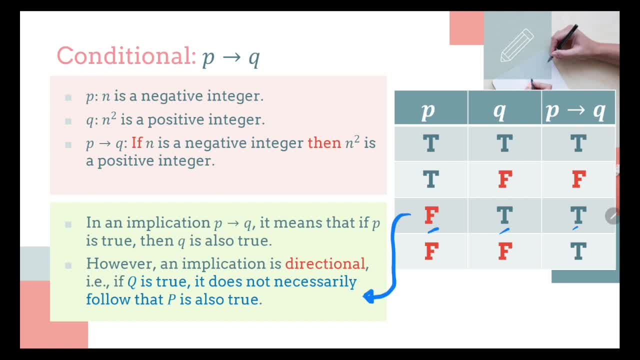 necessarily follow that P is also true. so Pwede siya false. that's why the so Pwede siya false. that's why the so Pwede siya false. that's why the teal true and when they are both false. teal true and when they are both false. 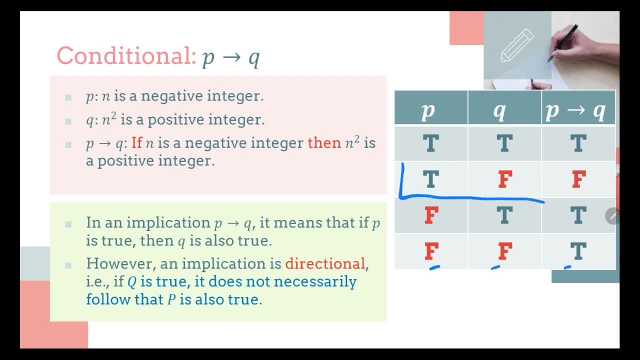 teal true, and when they are both false, then it is true. so you only have to take, then it is true. so you only have to take, then it is true. so you only have to take note of this one now, once your P is, note of this one now, once your P is. 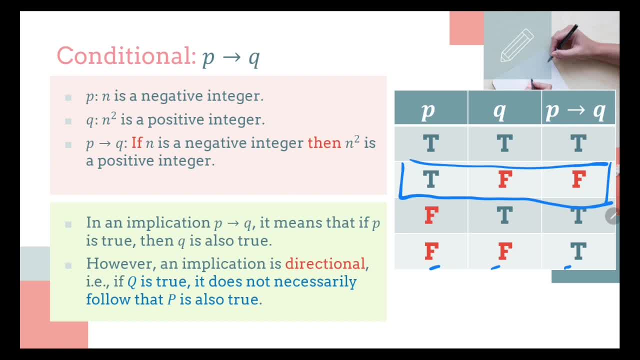 note of this one now, once. your P is true and your Q is false. that's the only true and your Q is false. that's the only true and your Q is false. that's the only time that your conditional statement is time that your conditional statement is. 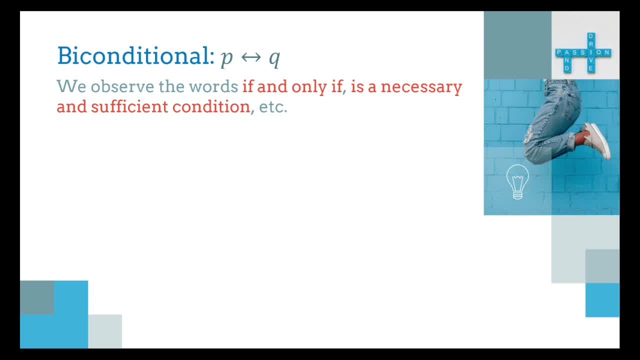 time that your conditional statement is false. by conditional. you serve the words false by conditional. you serve the words false by conditional. you serve the words if and only if is a necessary and if and only if is a necessary, and if and only if is a necessary and sufficient condition, etc. but usually if. 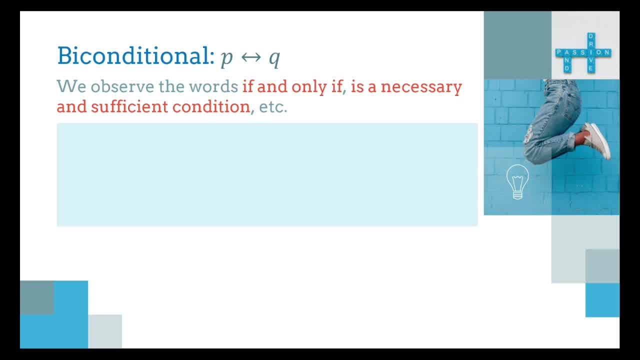 sufficient condition, etc. but usually if sufficient condition, etc. but usually if and only if- exam example: I will, and only if exam example: I will, and only if exam example: I will. graduate on time Q, I will pass all the. graduate on time Q, I will pass all the. 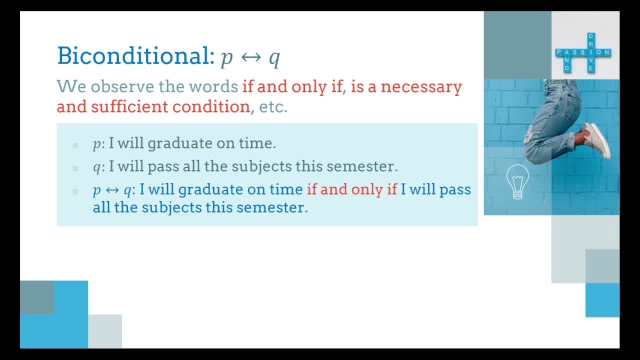 graduate on time. Q- I will pass all the subjects this semester. so I will subjects this semester. so I will subjects this semester. so I will graduate on time if and only if I will graduate on time, if and only if I will graduate on time if and only if I will pass all the subjects this semester. 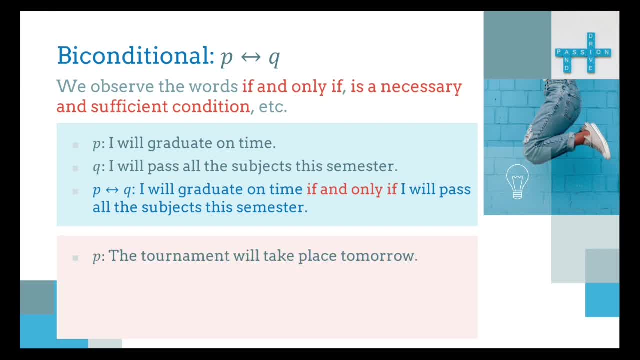 pass all the subjects this semester. pass all the subjects this semester. another one. the tournament will take another one. the tournament will take another one. the tournament will take place tomorrow. the weather is due place tomorrow. the weather is due place tomorrow. the weather is due, so the tournament will take place. 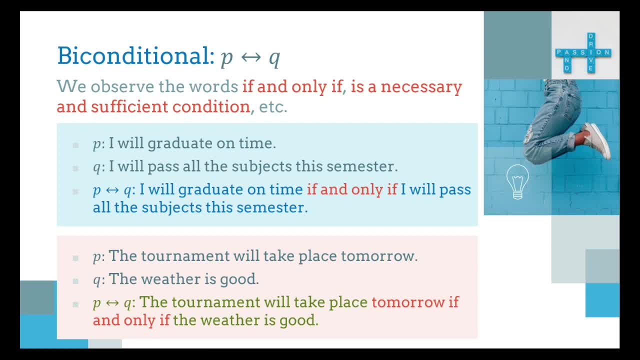 so the tournament will take place. so the tournament will take place tomorrow if and only if the weather is tomorrow. if and only if the weather is tomorrow, if and only if the weather is good. if the by conditional is true, we good. if the by conditional is true, we. 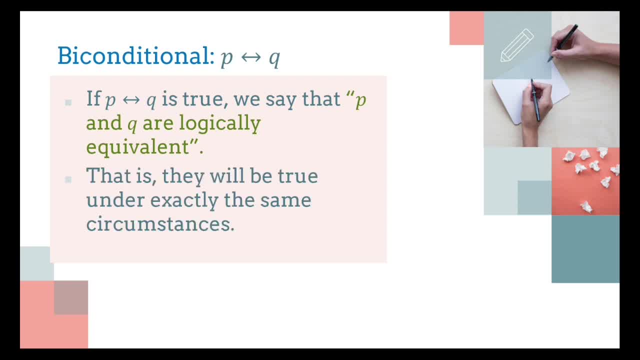 good if the by conditional is true. we say that P and Q are logically equivalent. say that P and Q are logically equivalent. say that P and Q are logically equivalent. that is, they will be true under exactly that is they will be true under exactly that is they will be true under exactly the same circumstances. so if you look at 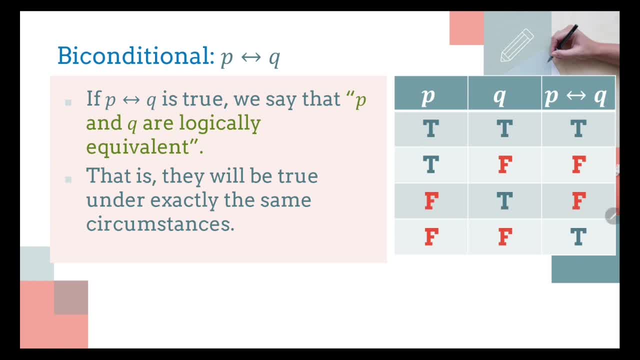 the same circumstances. so if you look at the same circumstances, so if you look at the truth table, if P and Q are true, it the truth table. if P and Q are true, it the truth table. if P and Q are true, it is true. true and false. false if false. 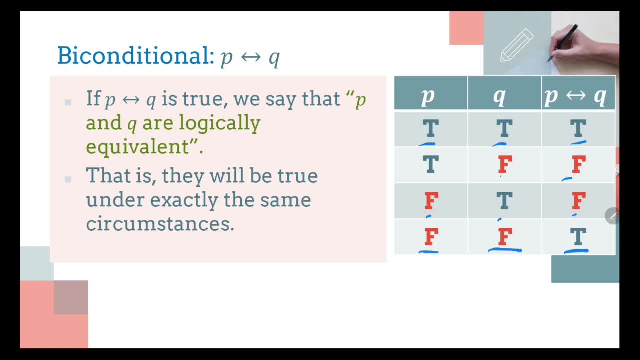 is true. false if false. false if false. true it's false. if they are both false, true it's false. if they are both false, true it's false if they are both false. it is true: P and Q should have the same. it is true: P and Q should have the same. 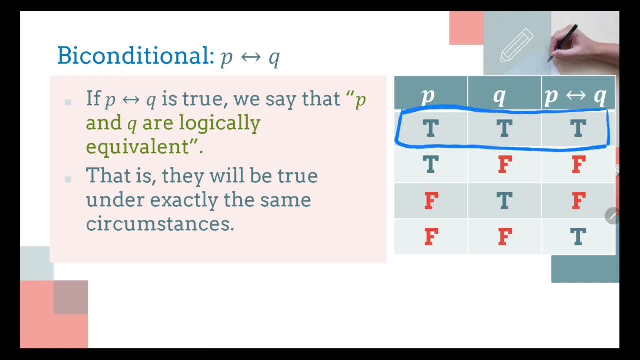 it is true. P and Q should have the same truth value for the by conditional to truth, value for the by conditional to truth, value for the by conditional to become true, so true. true to give out the become true, so true. true to give out the become true, so true. true to give out the true. if they are both false, then the. 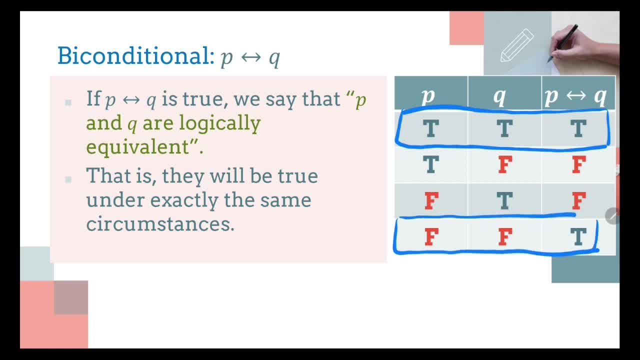 true. if they are both false, then the true. if they are both false, then the by conditional is also true. so you take by conditional is also true. so you take by conditional is also true. so you take note of this too. let's translate each of note of this too. let's translate each of. 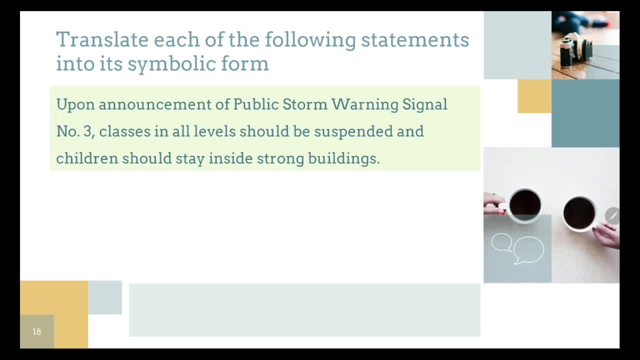 note of this too. let's translate each of the following statements into its: the following statements into its: the following statements into its symbolic form: upon announcement of symbolic form. upon announcement of symbolic form: upon announcement of public storm warning- signal number three: public storm warning signal number three: 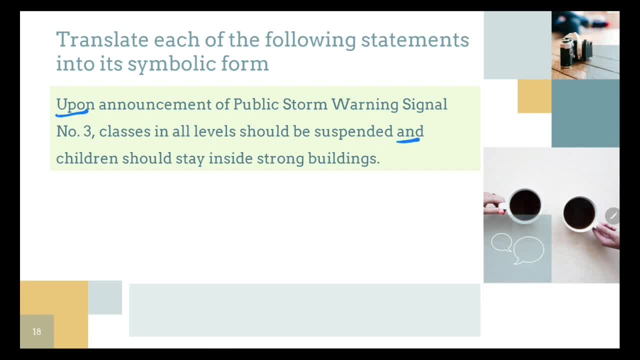 public storm warning signal number three: classes in all levels should be. classes in all levels should be. classes in all levels should be suspended and children should stay suspended and children should stay suspended and children should stay inside strong buildings. so if we inside strong buildings, so if we 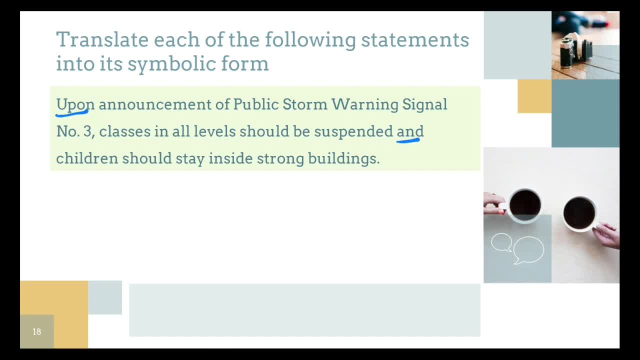 inside strong buildings. so if we analyze this, we have connectives upon analyze this, we have connectives upon analyze this, we have connectives upon and, and then the statements is somewhat, and, and then the statements is somewhat, and and then the statements is somewhat, divided into three parts. so the first, 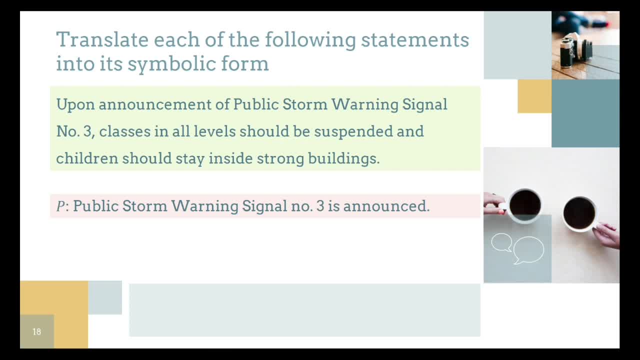 divided into three parts. so the first divided into three parts. so the first statement: public storm warning signal statement. public storm warning signal statement. public storm warning signal number three is announced, then we also number three is announced, then we also number three is announced, then we also have classes in all levels are suspended. 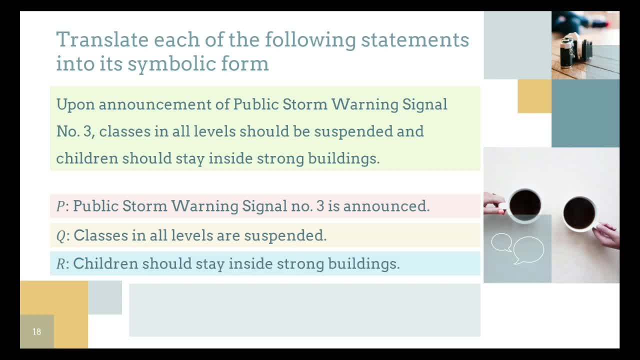 have classes in all levels are suspended, have classes in all levels are suspended, then we also have children should stay. then we also have children should stay. then we also have children should stay inside strong buildings. now looking back inside strong buildings, now looking back inside strong buildings. now looking back, we have the upon that would give us a. 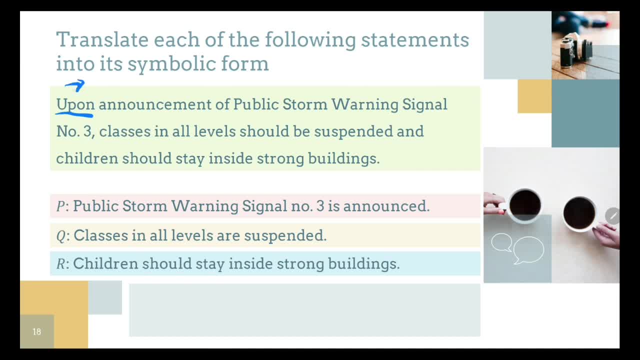 we have the upon that would give us a. we have the upon that would give us a conditional statement, and then we also conditional statement, and then we also conditional statement, and then we also have the and which give us that have the and which give us that have the and which give us that conjunction. 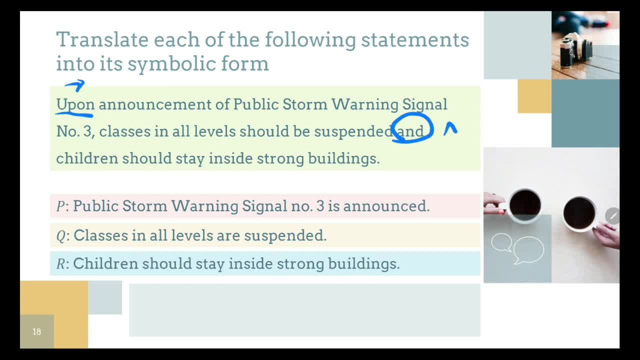 conjunction: conjunction. so combining the PQ and R, we have P then, so I cannot separate Q. so, combining the PQ and R, we have P then, so I cannot separate Q. so, combining the PQ and R, we have P then, so I cannot separate Q and R, so I will use. 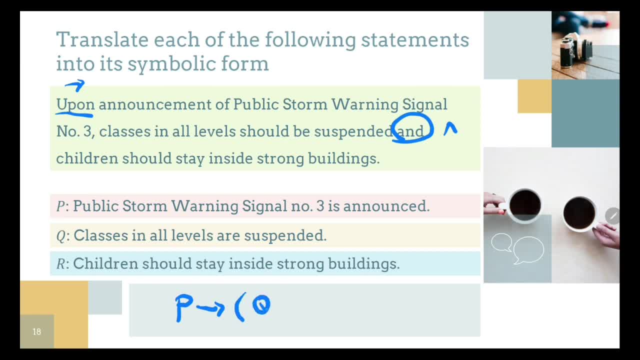 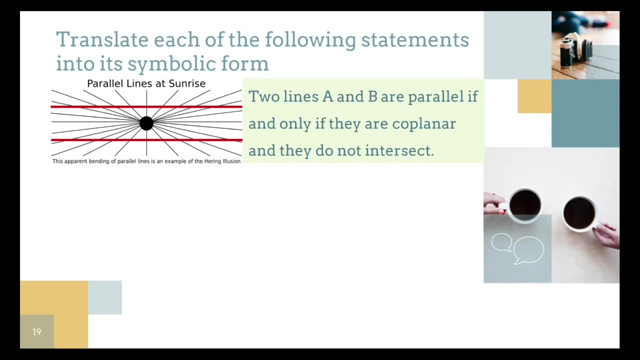 and R, so I will use and R, so I will use parentheses Q and it is a conjunction R. next two lines in next two lines, in next two lines in A and B are parallel if and only if they are. A and B are parallel if and only if they are. 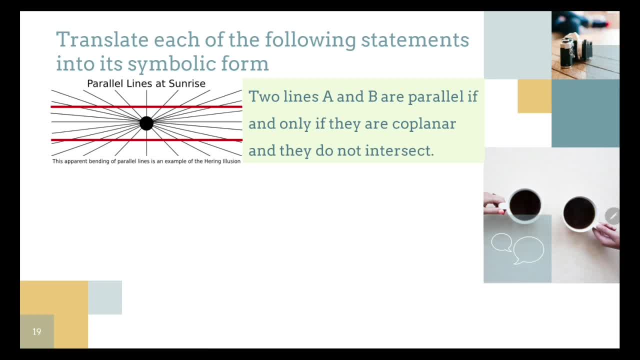 A and B are parallel, if and only if. they are coplanar and they do not intersect. so we coplanar and they do not intersect, so we coplanar and they do not intersect. so we have. if and only if, then we also have. have if and only if, then we also have. 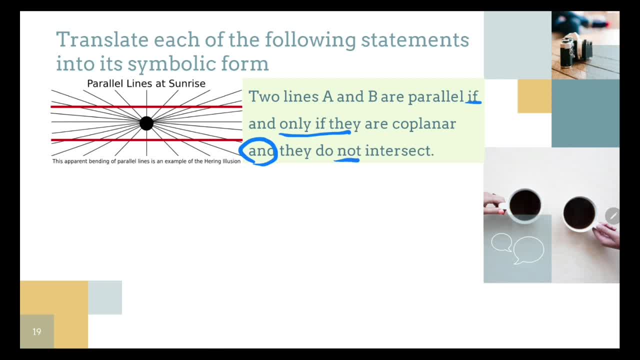 have if, and only if, then we also have the end here, and we also have the not the end here, and we also have the not the end here and we also have the not okay. so we also have here three okay. so we also have here three okay. so we also have here three statements. 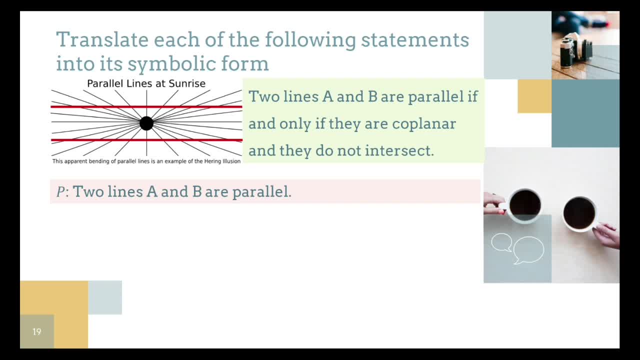 statements. okay, so we also have here three statements start with P. two lines, A and B, are start with P. two lines, A and B, are start with P. two lines- A and B are parallel lines A and B are coplanar, and parallel lines A and B are coplanar and. 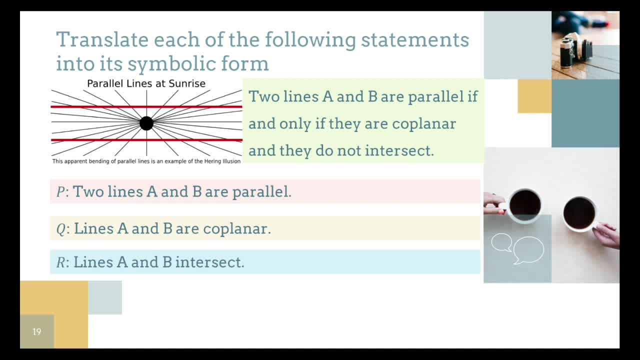 parallel lines A and B are coplanar and lines A and B intersect. so if I'm going lines A and B intersect, so if I'm going lines A and B intersect, so if I'm going to write the symbol I have here if, and to write the symbol I have here if and 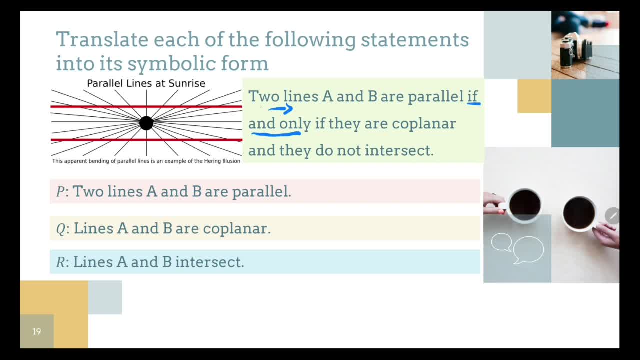 to write the symbol I have here: if and only if so. that would give me the only if so, that would give me the only if so. that would give me the biconditional, the symbol, biconditional, the symbol, biconditional, the symbol. I have the end. so I also have conjunction. 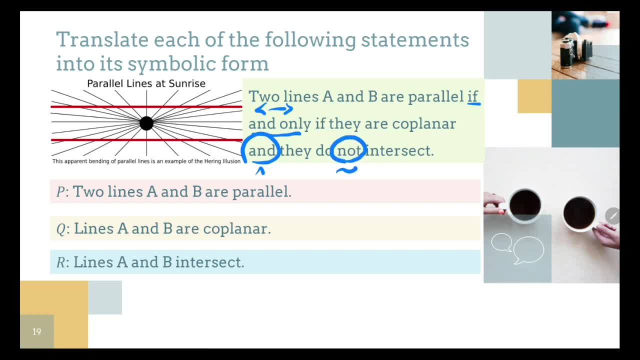 I have the end, so I also have conjunction. I have the end, so I also have conjunction. there is the not here, so I might negate. there is the not here, so I might negate. there is the not here, so I might negate statement R, so that would give me P if. 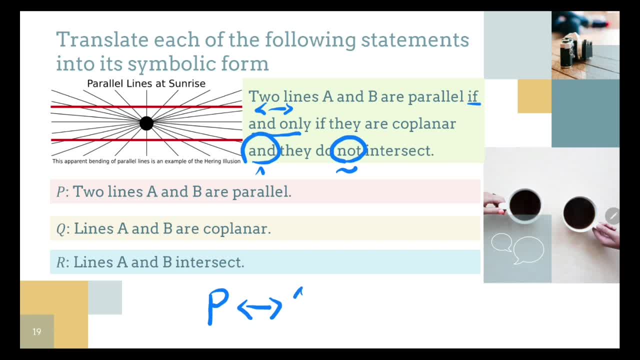 statement R, so that would give me P if. statement R, so that would give me P if, and only if, I have Q, and of course I'm, and only if I have Q, and of course I'm, and only if I have Q, and of course I'm going to negate our truth. tables of 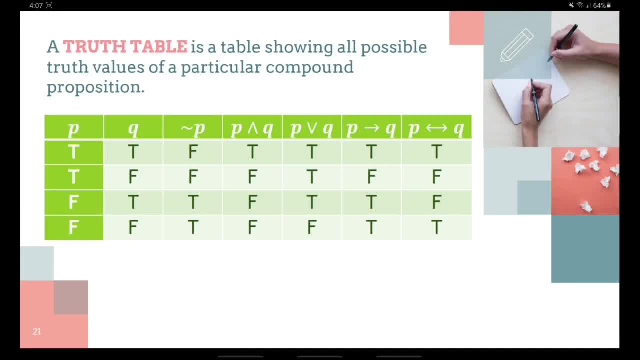 going to negate our truth. tables of going to negate our truth, tables of compound propositions. so I told this will compound propositions. so I told this will compound propositions. so I told this will be the summary of all of the truth. be the summary of all of the truth. 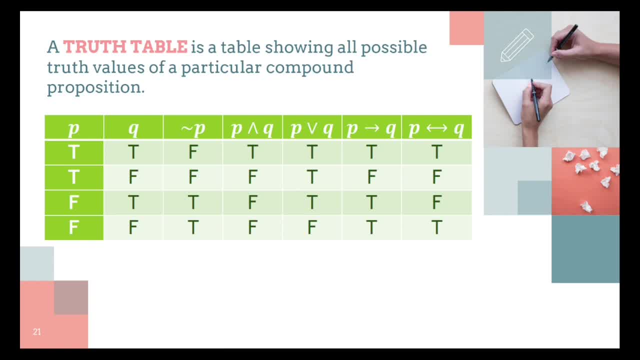 be the summary of all of the truth people, from negation to by conditional people, from negation to by conditional people, from negation to by conditional. so a truth people is a table showing all. so a truth people is a table showing all. so a truth people is a table showing all possible truth values of a particular 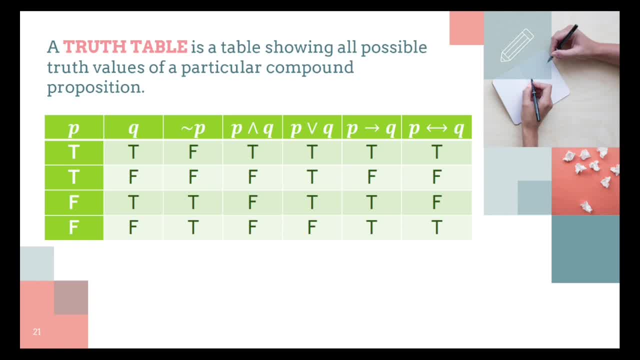 possible truth values of a particular possible truth values of a particular compound propositions. so we have here the compound propositions. so we have here the compound propositions. so we have here the summary. we have here the negation, the summary. we have here the negation, the summary. we have here the negation, the conjunction, the disjunction, the. 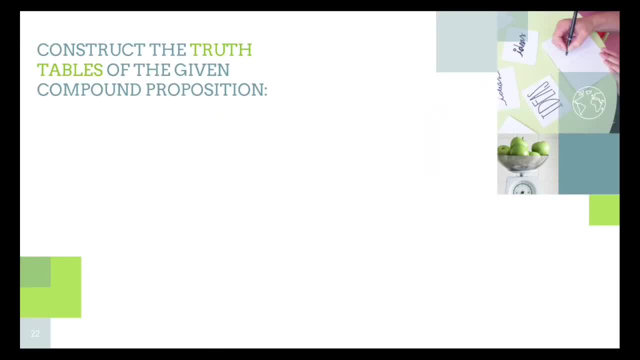 conjunction, the disjunction, the conjunction, the disjunction, the conditional, the by condition, and struck conditional, the by condition and struck conditional the by condition and struck the truth tables of the given compound. the truth tables of the given compound. the truth tables of the given compound. proposition: we have P and not P, since we 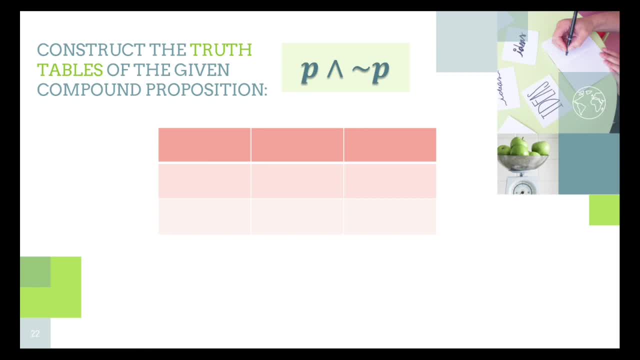 proposition we have P and not P. since we proposition we have P and not P, since we only have one variable which is P. so we only have one variable which is P. so we only have one variable which is P. so we only have two possible truth value, which: 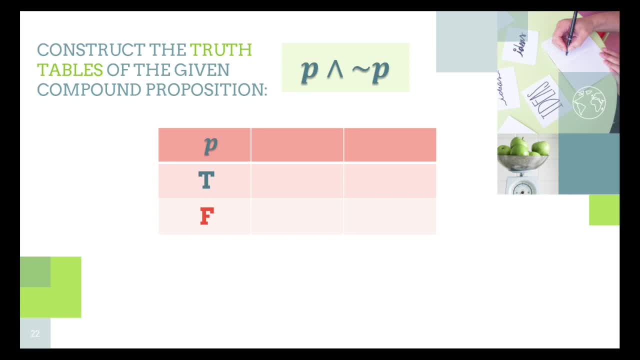 only have two possible truth value, which only have two possible truth value, which is true and false. so you find the not P is true and false. so you find the not P is true and false. so you find the not P so so, so true to become false from false and 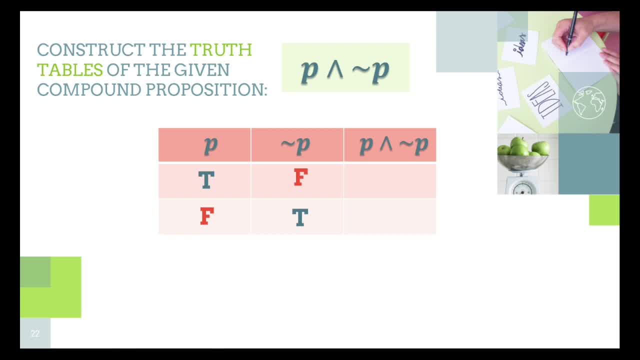 true to become false from false, and true to become false from false, and will become true, and then I'm going to will become true, and then I'm going to will become true, and then I'm going to find the conjunction of P and not P. if find the conjunction of P and not P, if 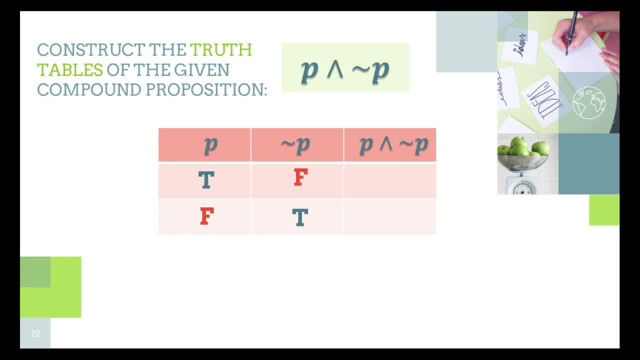 find the conjunction of P and not P if you recall for conjunction, the only time you recall for conjunction, the only time you recall for conjunction, the only time the statement is true. if they are both, the statement is true if they are both, the statement is true if they are both true. so true, false, false, false, true is. 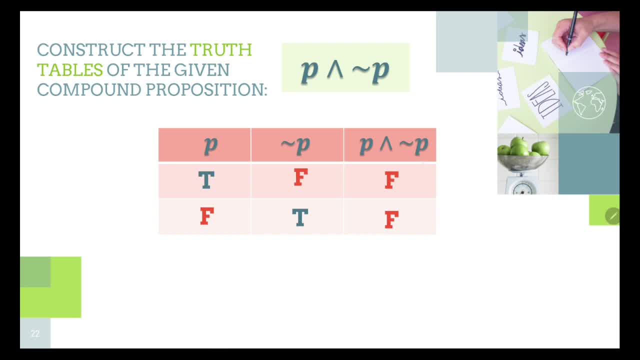 true, so true, false, false, false. true is true, so true, false, false, false. true is false. if all true value of your false, if all true value of your false, if all true value of your compound statement are all false, you compound statement are all false. you compound statement are all false. you, then we call this one a contradiction. 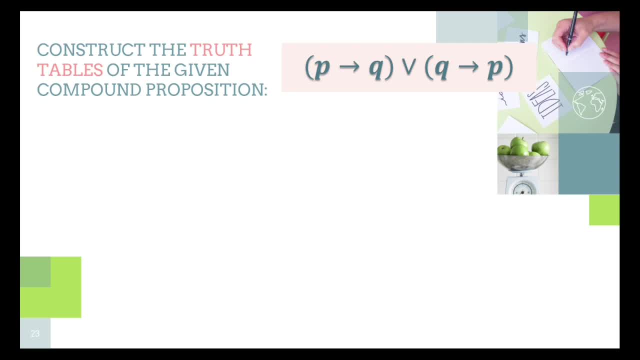 then we call this one a contradiction. then we call this one a contradiction. let's have this compound proposition. if let's have this compound proposition, if let's have this compound proposition, if P then Q, or if Q then P- in this case we- P then Q. or if Q then P- in this case we. 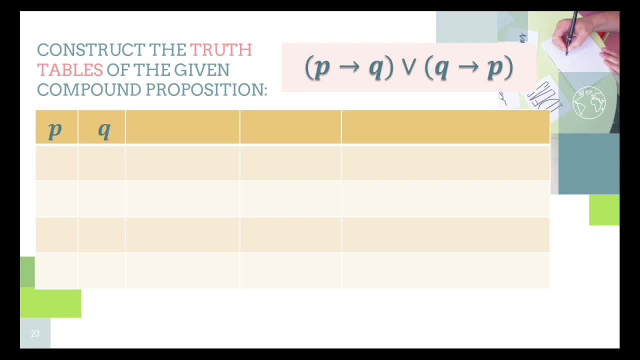 P then Q, or if Q then P. in this case we have two variables: P and Q. then we have have two variables, P and Q. then we have have two variables, P and Q. then we have four possible combination of their truth. four possible combination of their truth. 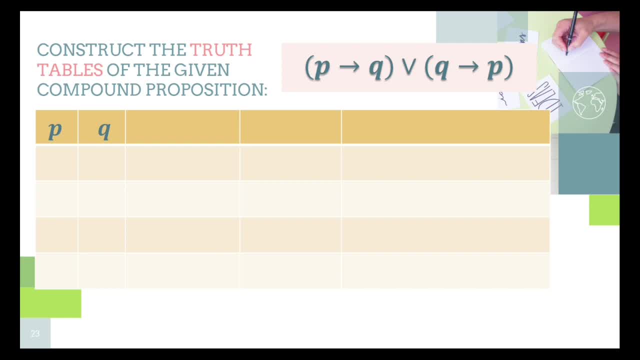 four possible combination of their truth, values, values, values, so so, so, so. so we have true, true, false, false, true, false, true, false, so both true. when one we have true, true, false, false, true, false, true, false, so both true. when one we have true, true, false, false, true, false, true, false, so both true when one is false and they are both false. next we need 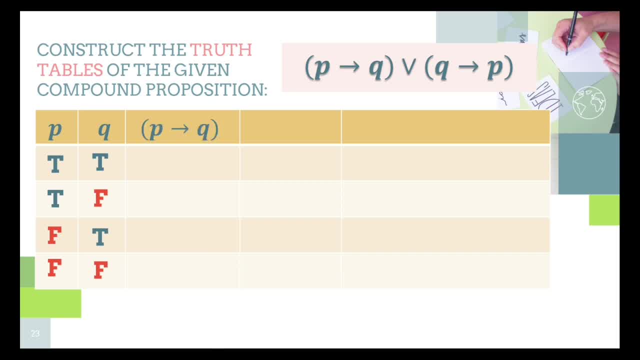 is false and they are both false. next, we need is false, and they are both false. next, we need to find the conditional statement P. to find the conditional statement P, to find the conditional statement P then Q, then we also need the Q then P, and then we also need the Q then P, and 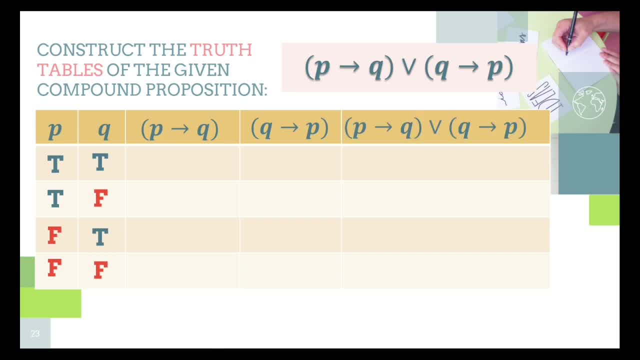 then we also need the Q, then P, and then we combine the two. so let's start with. then we combine the two. so let's start with, then we combine the two. so let's start with the conditional: if P, then Q, so the conditional: if P, then Q, so 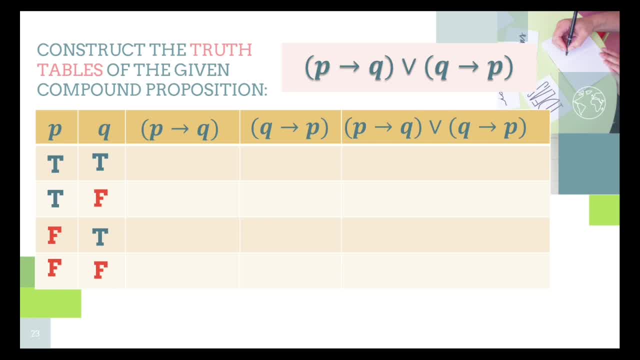 the conditional. if P, then Q, so for conditional, you have to remember the. for conditional, you have to remember the. for conditional you have to remember the only time that it will become false is only time that it will become false. is only time that it will become false is when you have a true first statement. 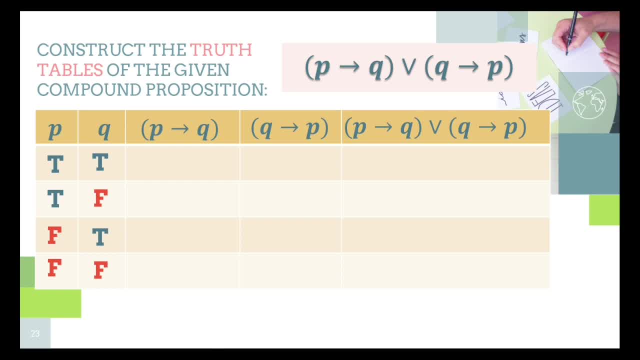 when you have a true first statement. when you have a true first statement, then it will give out a false consequent, then it will give out a false consequent, then it will give out a false consequent. so true, true, it's true, true and false. so true, true, it's true, true and false. 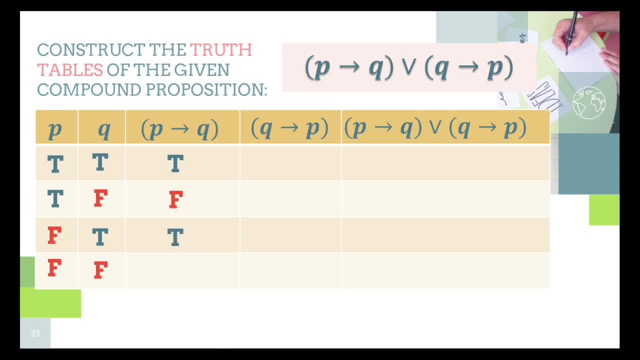 so true, true it's true, true and false it's false, false, true it's true. and if it's false, false, true it's true. and if it's false, false, true it's true. and if they are both false, true, they are both false, true they are both false, true. next, 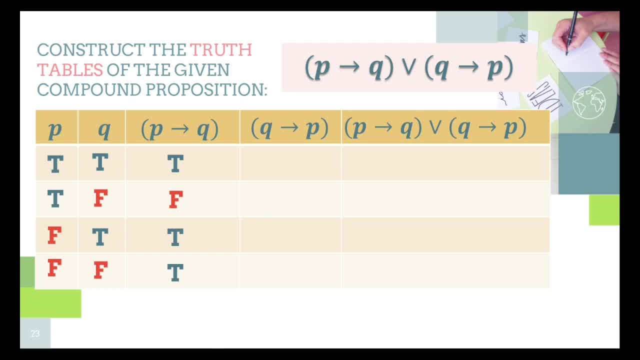 next, next, next. if Q, then P, so this time the only time it. if Q, then P, so this time, the only time it. if Q, then P, so this time. the only time it will become false is when your Q is true will become false is when your Q is true. 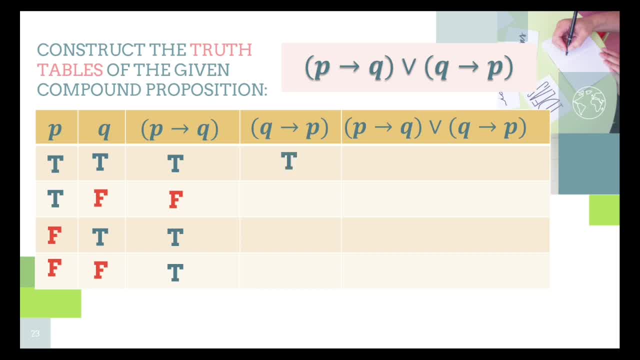 will become false is when your Q is true and your P is false, so true, then it's. and your P is false, so true then it's. and your P is false, so true, then it's. time it's true, false, and then we are time it's true, false and then we are. 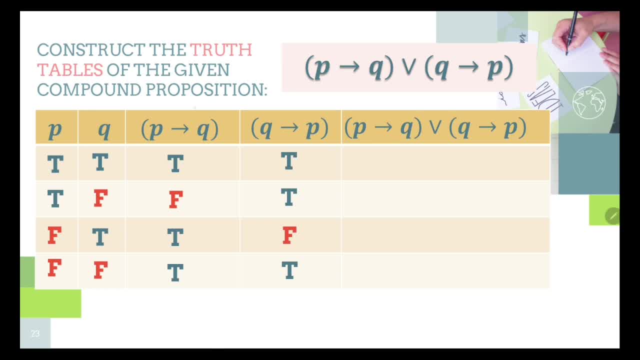 time it's true, false, and then we are going to look at this two columns- okay, going to look at this two columns. okay, going to look at this two columns. okay, we're going to combine this two. we're going to combine this two. we're going to combine this two, okay. 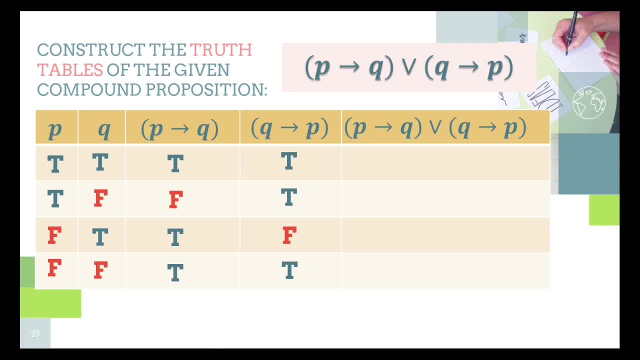 okay, okay, so, or for this junction, the only time it so, or for this junction the only time it so, or for this junction the only time it will become false, since when they are will become false, since when they are, will become false, since when they are both false. so, true, true, it's true, false. 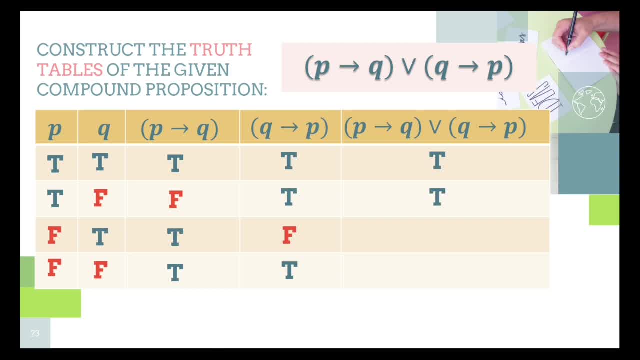 both false, so true. true it's true, false. both false, so true. true it's true. false or true is true. true or false is also. or true is true, true or false is also. or true is true, true or false is also true, and true or true is also true when. 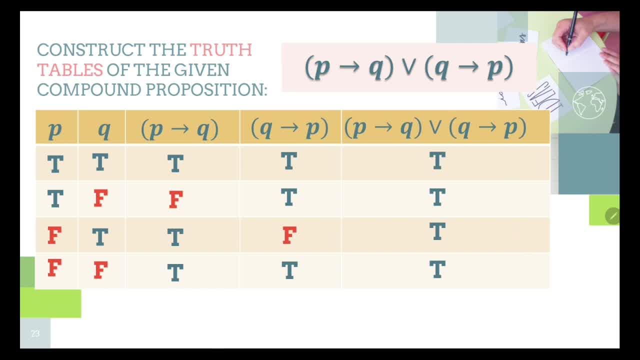 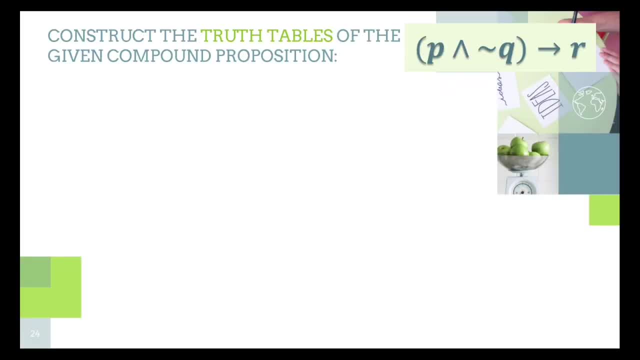 true and true or true is also true. when true and true or true is also true. when all your truth value are all true, call all your truth value are all true. call all your truth value are all true. call this, this, this one at the top of the G. next we have P and not. you. then are in here we. 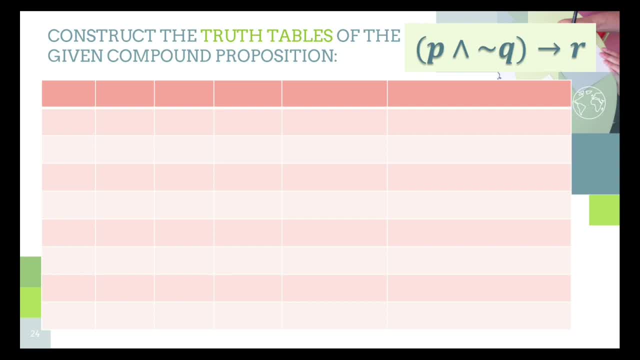 one at the top of the G, next we have P and not you. then are in here. we have one at the top of the G. next we have P and not you. then are in here. we have three variables: P, Q and R. so that would three variables: P, Q and R. so that would. 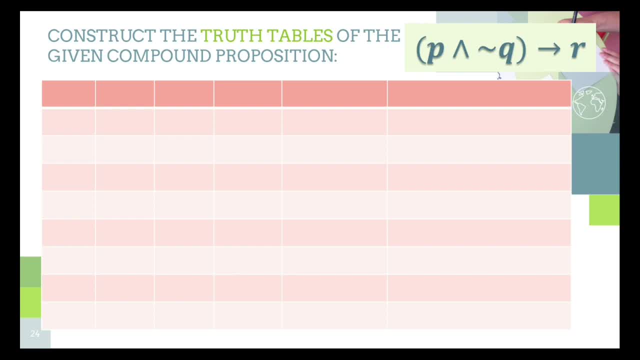 three variables: P, Q and R. so that would give us eight possible combinations of. give us eight possible combinations of, give us eight possible combinations of their true values. it's basically two, their true values. it's basically two, their true values. it's basically two times two times two. that's why we have 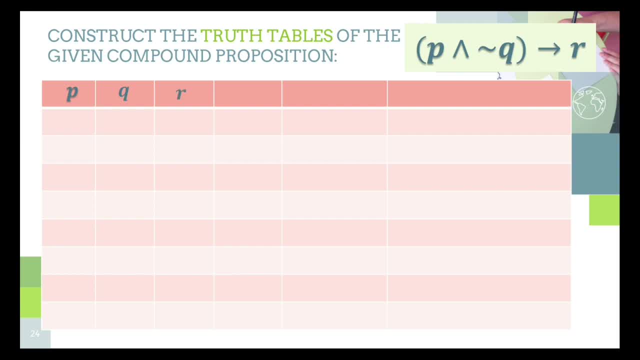 times two times two. that's why we have times two times two. that's why we have eight. so we need to find P, Q and eight. so we need to find P, Q and eight. so we need to find P, Q and our combinations, and then we also need not. 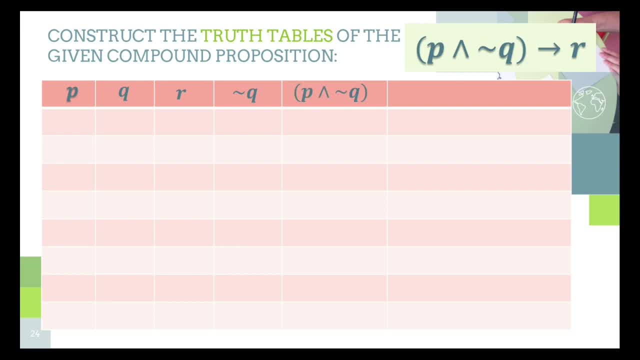 our combinations, and then we also need not our combinations, and then we also need not Q. then we combine it with P and not Q, then we combine it with P and not Q, then we combine it with P and not Q, and then we have the conditional P and 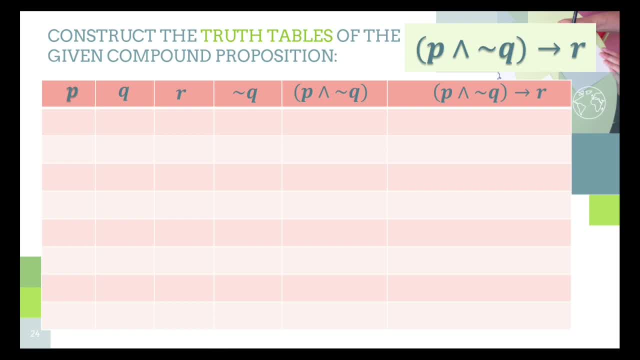 Q, and then we have the conditional P and Q, and then we have the conditional P and Q. then are so to find the combinations Q, then are so to find the combinations Q. then are so to find the combinations of PQ. re can follow this pattern true of PQ. re can follow this pattern true. 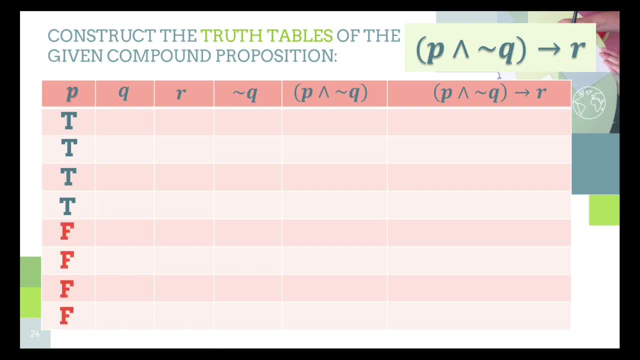 of PQ re can follow this pattern: true, true, true, true, false, false, false, false, true, true, true, true, false, false, false, true, true, true, true, false, false, true, true, false, false, and then true, true, true, false, false, true, true, false, false, and then true, true, true, false, false, true, true, false, false, and then true, false, false and then true. 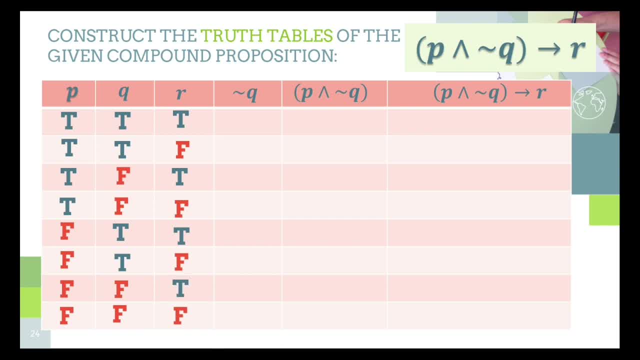 false, false, false, and then true, false, false, and then true, false, false, false, true, false, true, false, false, false, true, false, true, false, true, false, false, false, all right. so next for false: false: all right, so next for false false. all right, so next for the thought Q. so we only have to look at: 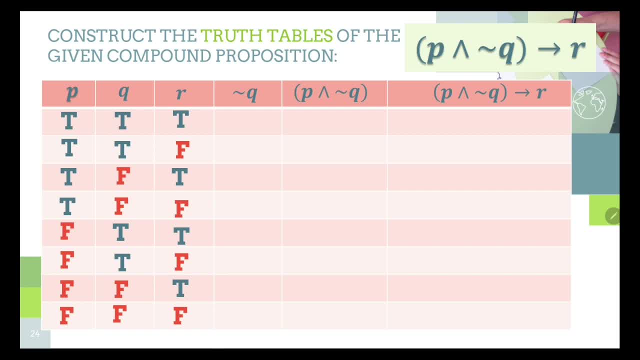 the thought Q. so we only have to look at the thought Q. so we only have to look at this column: so false, false, true, true this column. so false, false, true, true this column. so false, false, true, true, false, false, true, true. and then we're false, false, true, true, and then we're. 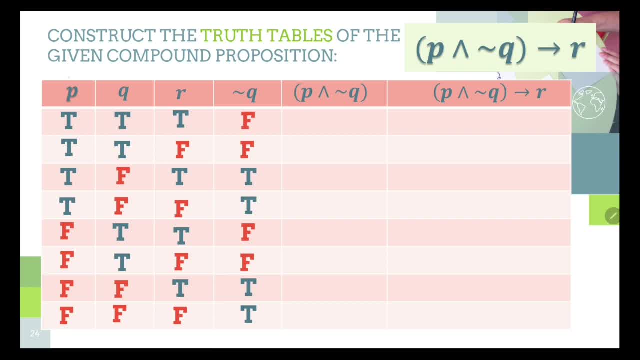 false, false, true, true. and then we're going to combine P this column and the going to combine P this column and the going to combine P this column and the not Q, not Q, not Q. so we're only going to look at this two. so we're only going to look at this two. 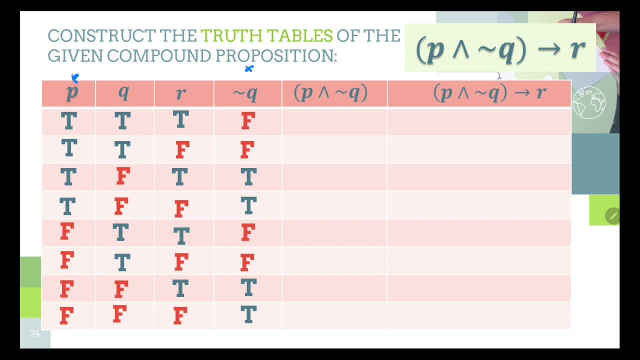 so we're only going to look at this: two column and it is a conjunction. so it column and it is a conjunction. so it column and it is a conjunction. so it should be both true to make the should be both true to make the. should be both true to make the statement true. so true, false, false, true. 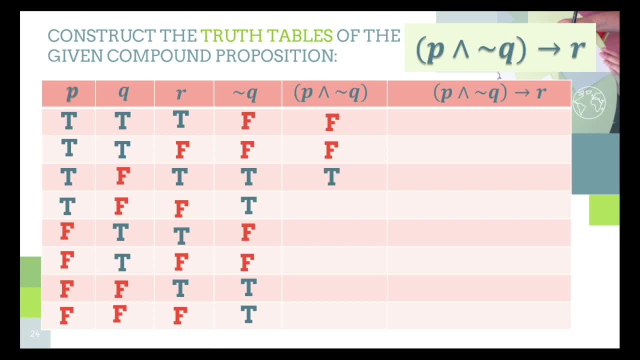 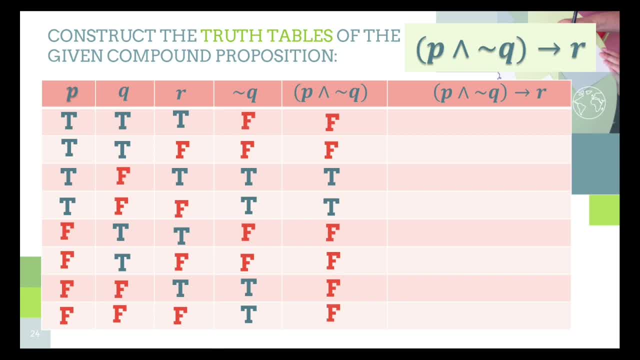 true, true is false, false, false, false, false, false true is false, false and false true is also false, false, false, true is also false, false, false, false true is also false. and then we have conditional false, and then we have conditional false, and then we have conditional statement, this column and this column. so 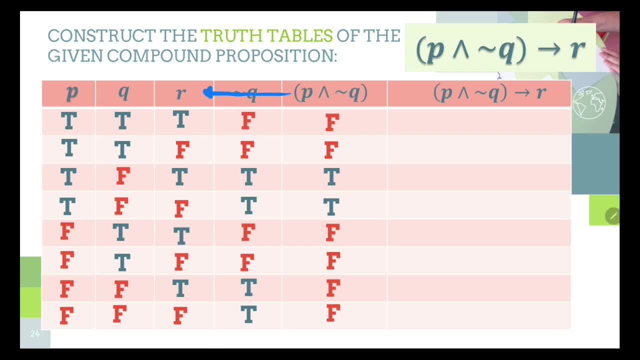 statement this column and this column. so, statement this column and this column. so we're going to combine this two. you have, we're going to combine this two. you have, we're going to combine this two. you have to remember for conditional statements, to remember for conditional statements. 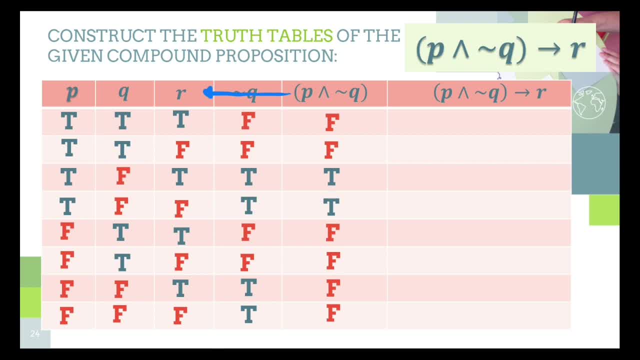 to remember, for conditional statements. the only time it will become false is the only time it will become false is the only time it will become false is when you have a true, then false. so when you have a true, then false. so when you have a true, then false, so false. true is true, false, false is true. 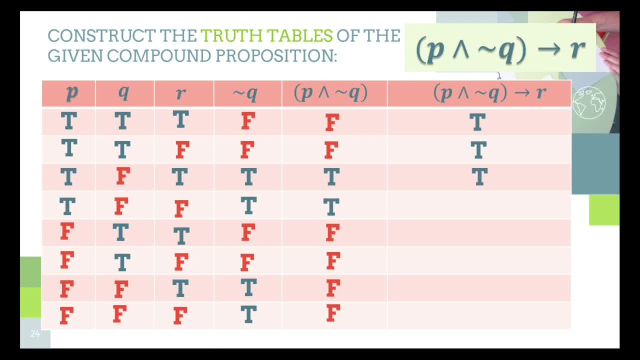 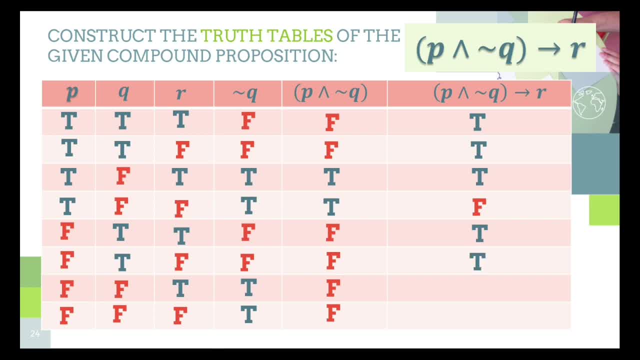 it's false, false, true is true. false, false is true. false, true is true, false is true. false, false is true. false, true is true. false, false is true. so if you have false, false is true. so if you have false, false is true. so if you have this kind of. 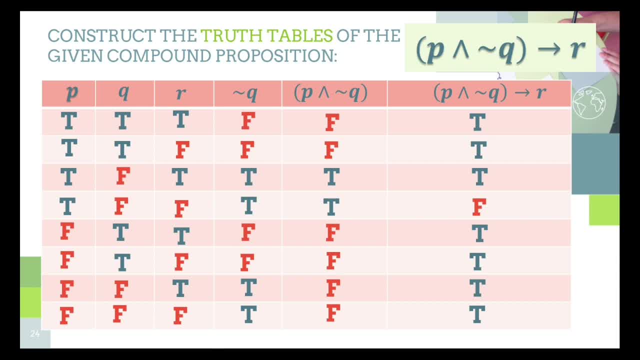 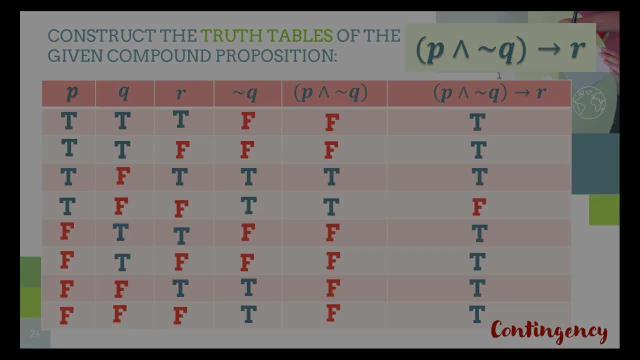 this kind of, this kind of compound proposition, which is a mix of true compound proposition, which is a mix of true compound proposition, which is a mix of true and false, then we call this one a and false, then we call this one a and false, then we call this one a contingency. so tautology, contradiction. 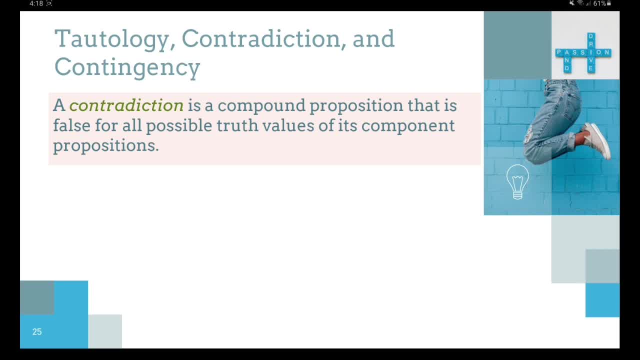 contingency, so tautology contradiction, contingency, so tautology, contradiction and contingency. so a contradiction is a and contingency. so a contradiction is a and contingency, so a contradiction is a compound proposition. that is false for compound proposition. that is false for compound proposition. that is false for all possible truth values of its. 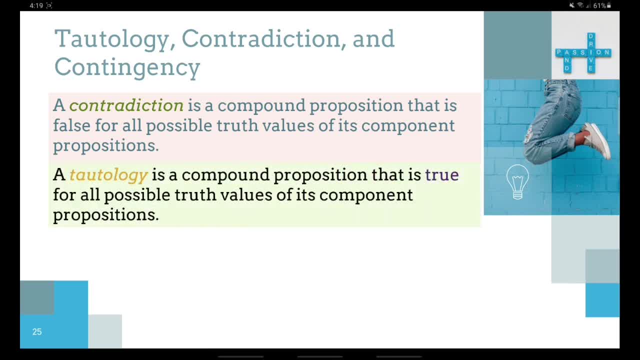 all possible truth values of its all possible truth values, of its component propositions. a tautology is a component propositions. a tautology is a component propositions. a tautology is a compound proposition. that is true for compound proposition. that is true for compound proposition. that is true for all possible truth values and all possible. 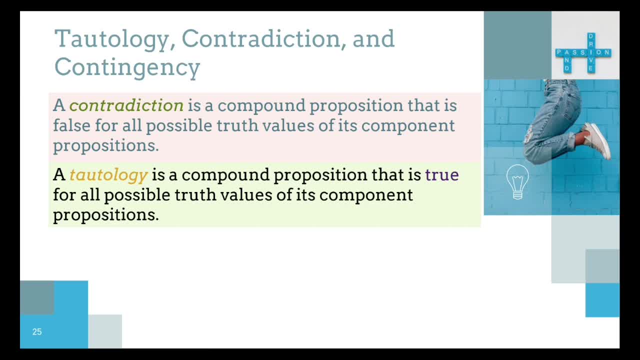 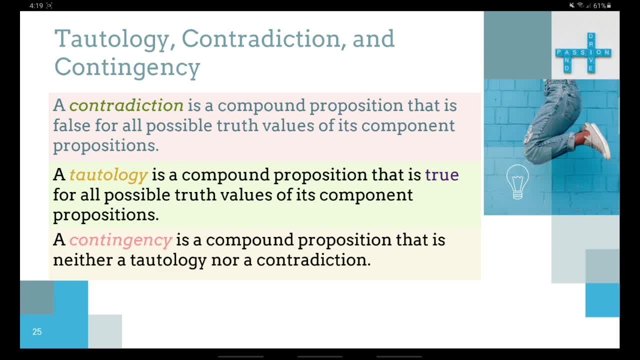 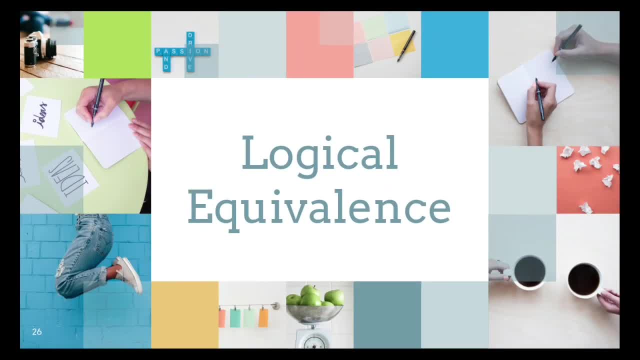 it's the opposite of the contradiction and a contingency is a contradiction and a contingency is a contradiction and a contingency is a compound proposition. that is neither a compound proposition. that is neither a compound proposition. that is neither a tautology nor a contradiction logical tautology nor a contradiction logical. 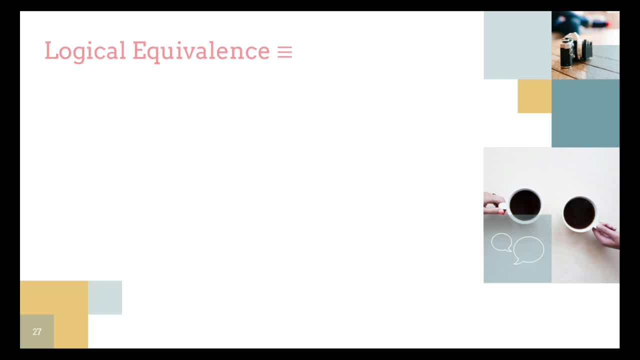 tautology, nor a contradiction. logical equivalence, so logical equivalence. we equivalence, so logical equivalence. we equivalence, so logical equivalence. we have that symbol. three lines, given any. have that symbol. three lines, given any. have that symbol. three lines, given any. compound compound propositions P and Q P. compound compound propositions P and Q P. 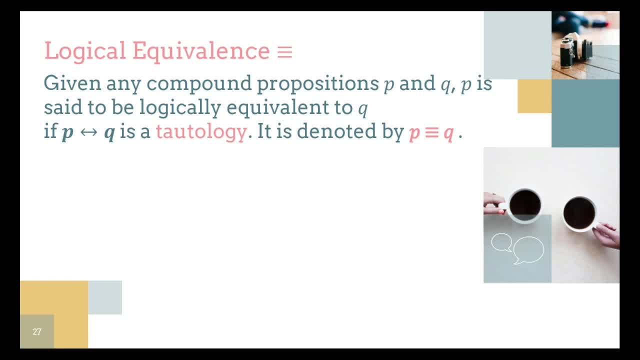 compound compound propositions P and Q. P is said to be logically equivalent to Q. is said to be logically equivalent to Q. is said to be logically equivalent to Q if the by conditional PQ is a tautology. if the by conditional PQ is a tautology. 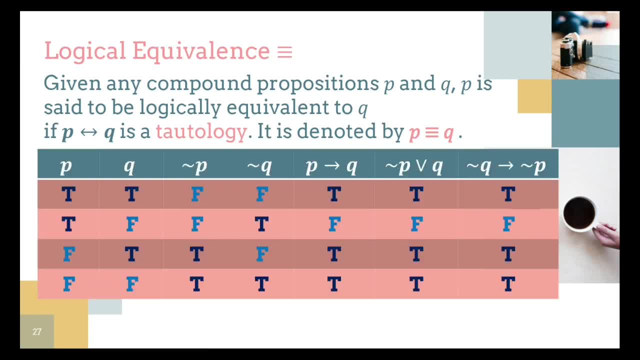 if the by conditional PQ is a tautology, is denoted by this. let's take a look at. is denoted by this. let's take a look at. is denoted by this. let's take a look at this example. if you notice, we have here. 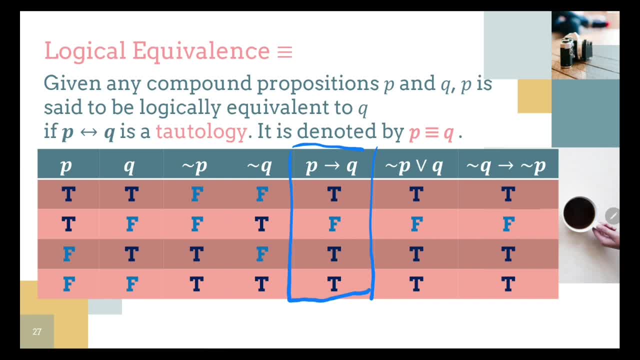 this example. if you notice we have here this example. if you notice, we have here the by conditional P, then Q. we also have the by conditional P, then Q. we also have the by conditional P, then Q. we also have another here, not P or Q, and here then 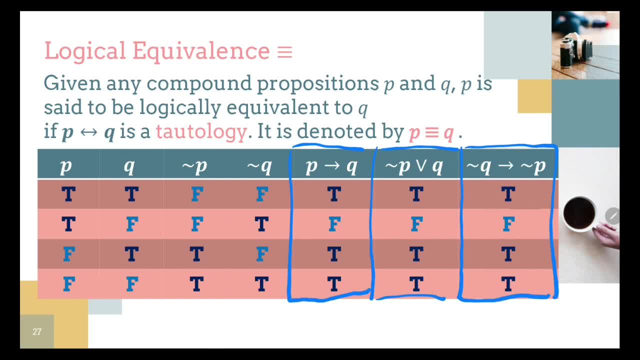 another: here not P or Q, and here. then another: here not P or Q, and here then not. if not Q, then not P, not. if not Q, then not P, not. if not Q, then not P. they are three different compound. they are three different compound. they are three different compound propositions, but their truth value are: 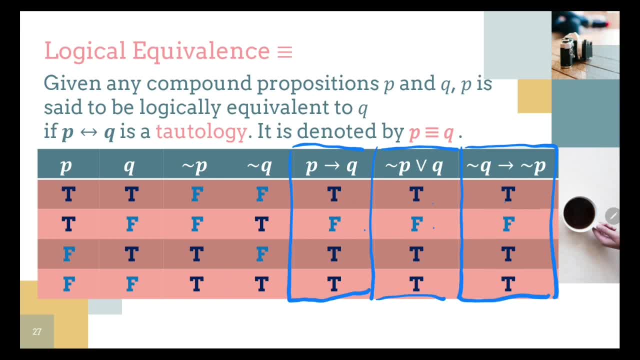 propositions, but their truth value are propositions, but their truth value are identical true, false, true, true, true, identical true, false, true, true, true, true, identical true, false, true, true, true, true, false, true, true. then we could say false, true, true, true. then we could say false true, true, true, true, true, false, true, true. then we could say that these three are: 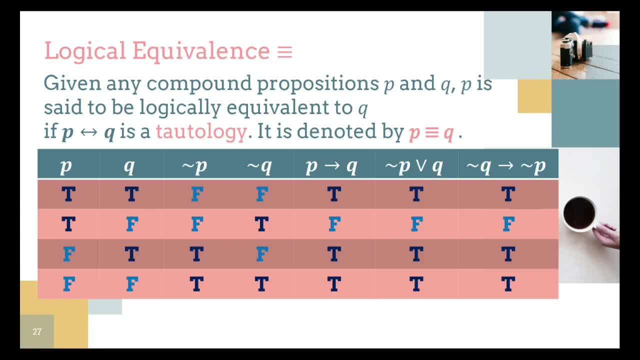 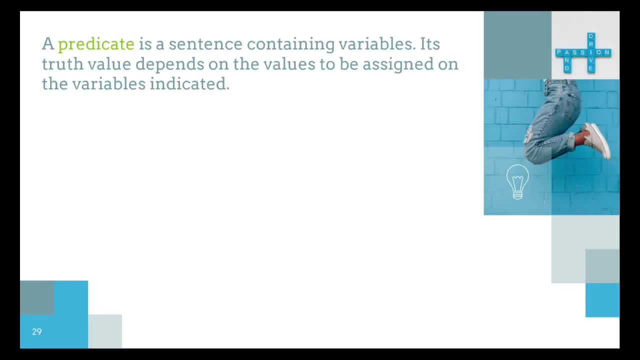 that these three are that these three are logically equivalent predicates and logically equivalent predicates and logically equivalent predicates and quantifiers. a predicate is a sentence. quantifiers. a predicate is a sentence. quantifiers. a predicate is a sentence contained. contained. contained variable. its truth value depends on the. 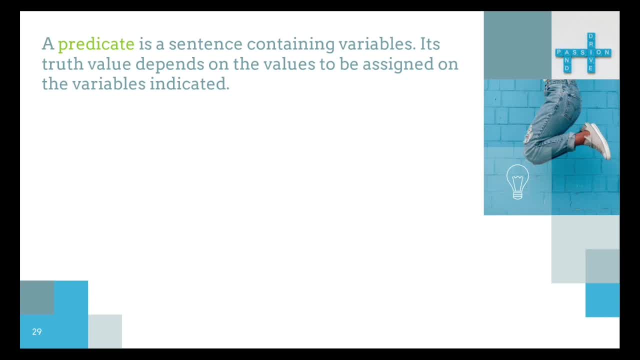 variable. its truth value depends on the variable. its truth value depends on the values to be assigned on the variables. values to be assigned on the variables. values to be assigned on the variables indicated. X is a real number, so we don't indicated. X is a real number, so we don't. 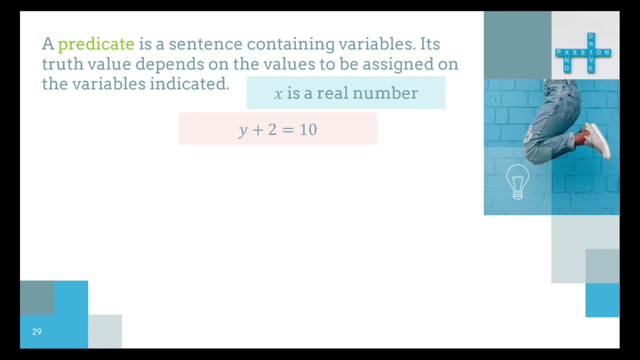 indicated X is a real number. so we don't know if this is true or false, unless we know if this is true or false. unless we know if this is true or false, unless we know the value of X, Y plus 2 is equal to know the value of X, Y plus 2 is equal to. 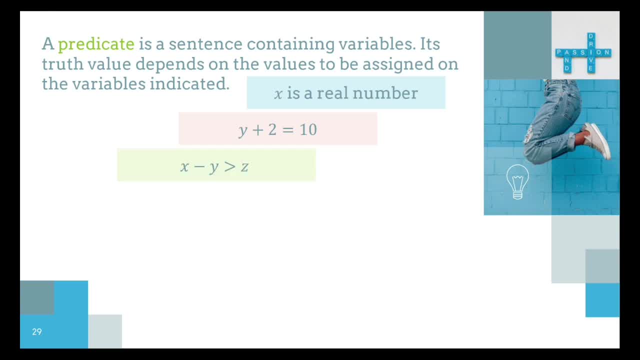 know, the value of X, Y plus 2 is equal to 10. X minus Y is greater than Z. a 10 X minus Y is greater than Z. a 10 X minus Y is greater than Z. a predicate is also known as. a predicate is also known as a. 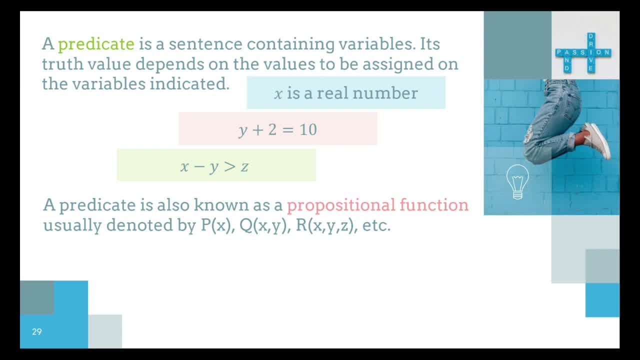 predicate is also known as a propositional function, usually denoted propositional function, usually denoted propositional function, usually denoted by P of X, Q, X, Y, R, X, Y, Z, etc. a by P of X, Q, X, Y, R, X, Y Z, etc. a by P of X, Q, X, Y, R, X, Y, Z, etc. a counter example is the value assigned to a. 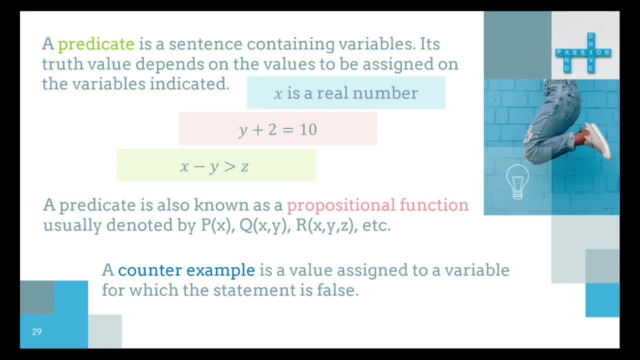 counter. example: is the value assigned to a counter. example: is the value assigned to a variable for which statement is false. variable for which statement is false. variable for which statement is false. once the value is assigned to variables, once the value is assigned to variables, once the value is assigned to variables, the predicate becomes a proposition with: 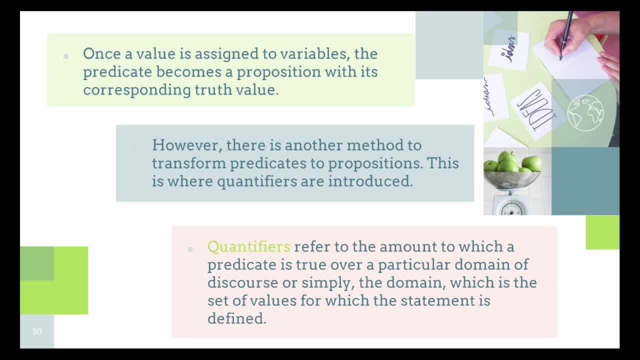 the predicate becomes a proposition, with the predicate becomes a proposition with its corresponding truth value, however, its corresponding truth value, however, its corresponding truth value. however, there is another method to transform. there is another method to transform. there is another method to transform predicates to propositions. this is where 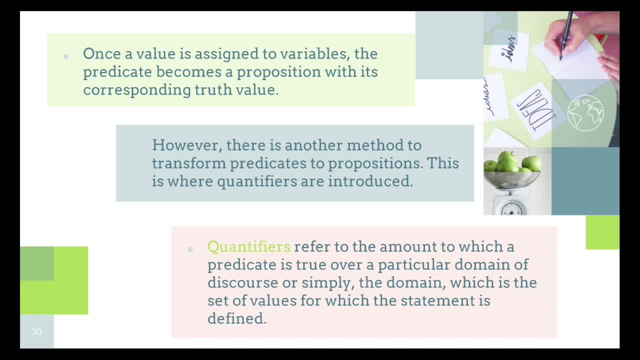 predicates to propositions. this is where predicates to propositions. this is where quantifiers are introduced. quantifiers, quantifiers are introduced. quantifiers, quantifiers are introduced. quantifiers. refers to the amount to reach a. refers to the amount to reach a. refers to the amount to reach a predicate is true over a particular. 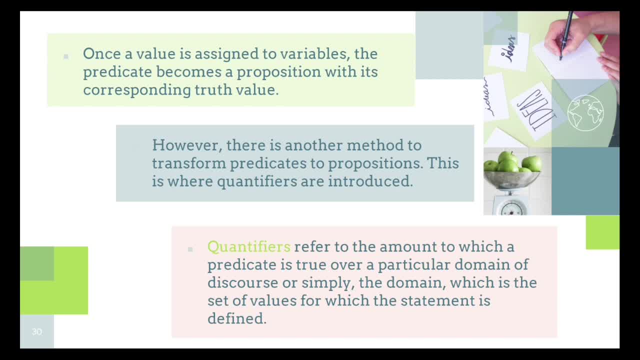 predicate is true over a particular predicate is true over a particular domain of discourse, or simply the domain domain of discourse, or simply the domain domain of discourse, or simply the domain, which is a set of values for which the which is a set of values for which the 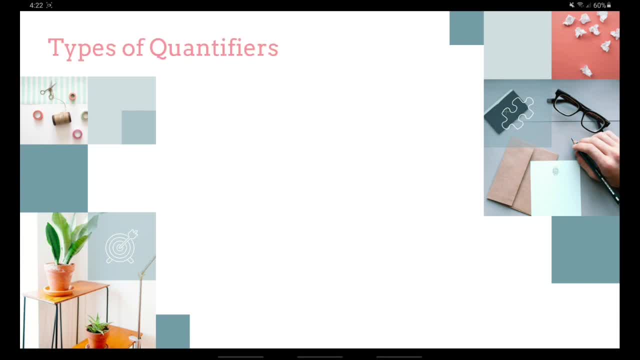 which is a set of values for which the statement is defined. so you have types. statement is defined, so you have types. statement is defined, so you have types of quantifiers. universal quantifier of quantifiers. universal quantifier of quantifiers. universal quantifier, denoted by this symbol, refers to the 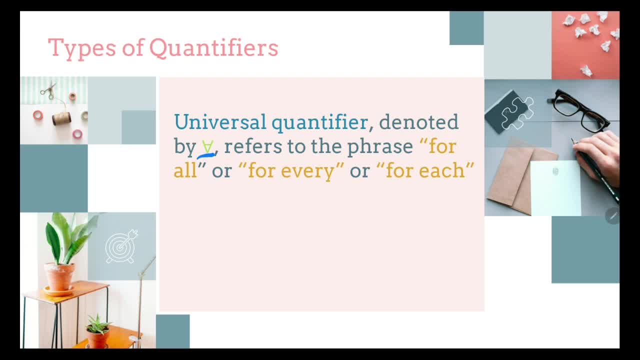 denoted by this symbol refers to the. denoted by this symbol refers to the phrase for all or for all. phrase for all or for all. phrase for all or for all, every or for each, every or for each, every or for each. example for all values of x. element of. 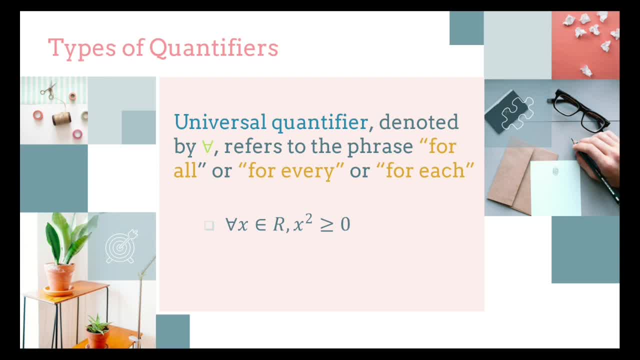 example, for all values of x. element of example. for all values of x. element of real numbers. x squared is greater than real numbers. x squared is greater than real numbers. x squared is greater than equal to zero. equal to zero. equal to zero. for all values of x, element of natural. 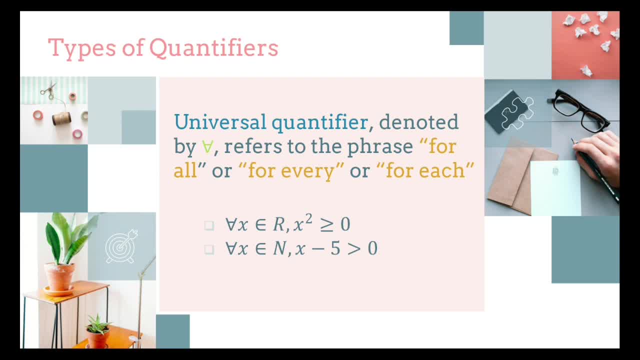 for all values of x element of natural. for all values of x element of natural. numbers x minus 5 is greater than zero. numbers x minus 5 is greater than zero. numbers x minus 5 is greater than zero. for all values of x and for all values. 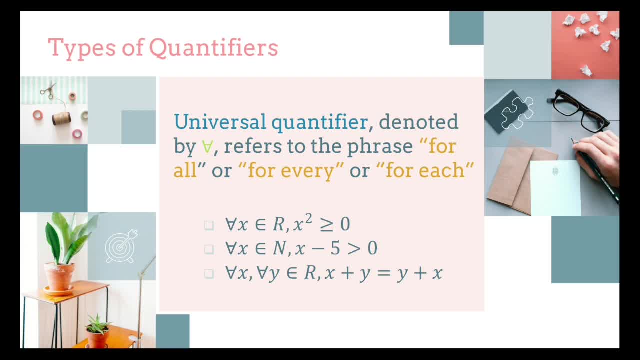 for all values of x and for all values, for all values of x and for all values of y, of y, of y, element of a real number. x plus y is element of a real number. x plus y is element of a real number. x plus y is equal to y plus x. 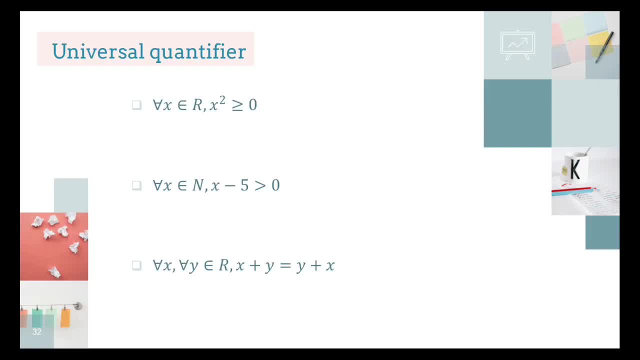 equal to y plus x. equal to y plus x. let's try to find the truth value of. let's try to find the truth value of. let's try to find the truth value of these, these, these statements, statements, statements for all values of x. element of r. 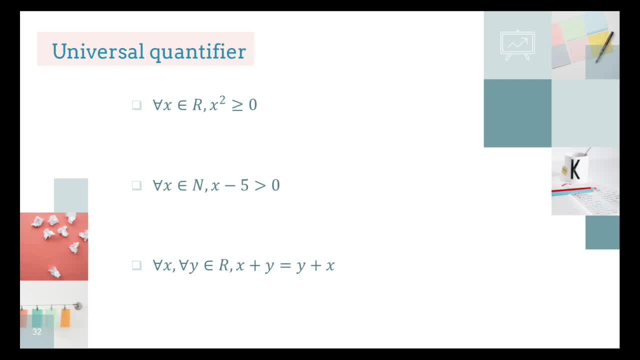 for all values of x element of r. for all values of x element of r. x squared is greater than zero. x squared is greater than zero. x squared is greater than zero. if you could find a counter example. if you could find a counter example, if you could find a counter example, our one value, that would make the 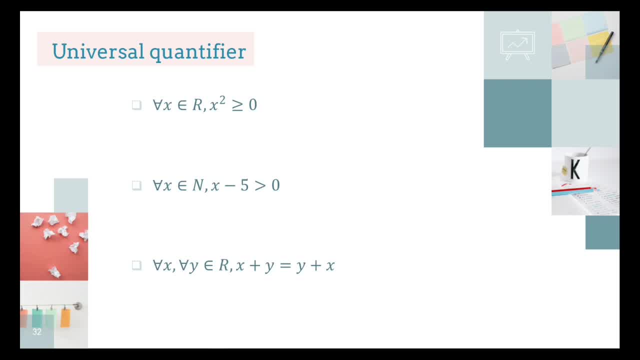 our one value. that would make the our one value. that would make the statement false, then the whole statement false, then the whole statement false, then the whole statement becomes false, statement becomes false, statement becomes false. but since i think we cannot, but since i think we cannot, but since i think we cannot find, 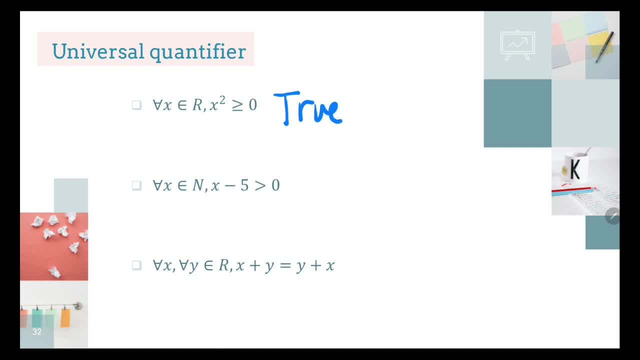 find, find. so i could say that this is a true, so i could say that this is a true, so i could say that this is a true statement. next for all values of x element of. next for all values of x, element of. next for all values of x. element of natural numbers. counting numbers one, two. 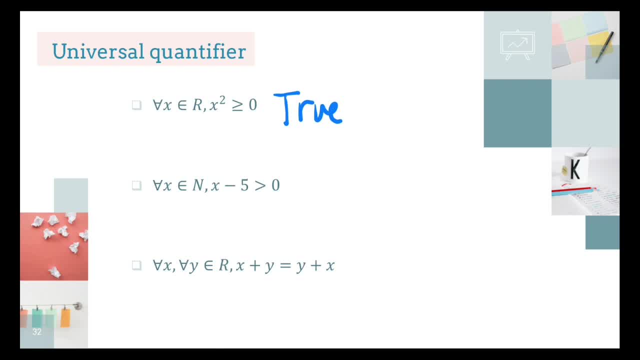 natural numbers counting numbers one, two. natural numbers counting numbers one, two, three, four, five, six, seven, eight, three, four, five, six, seven, eight, three, four, five, six, seven, eight x minus five is greater than zero. x minus five is greater than zero. x minus five is greater than zero. and this one is false. 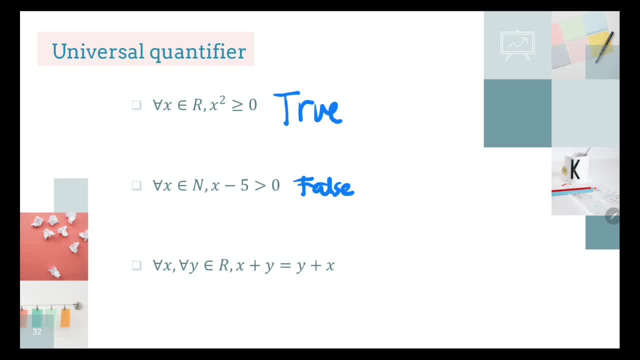 and this one is false and this one is false. okay, so to back up our okay, so to back up our okay, so to back up our answer that it is false, we need a answer that it is false. we need a answer that it is false. we need a counter example. 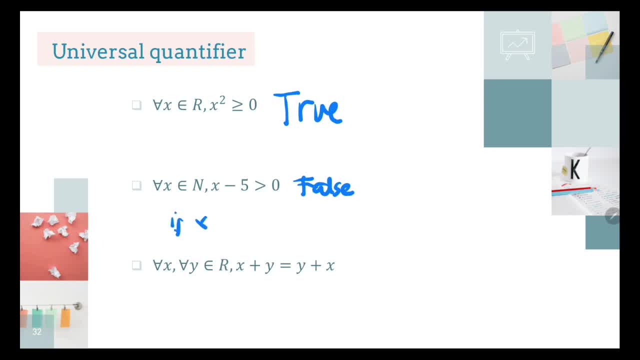 counter example, counter example. so i think, if your x is equal to so, i think, if your x is equal to so, i think, if your x is equal to one, maybe one, maybe one, maybe, okay, so that would give me one minus. okay, so that would give me one minus. 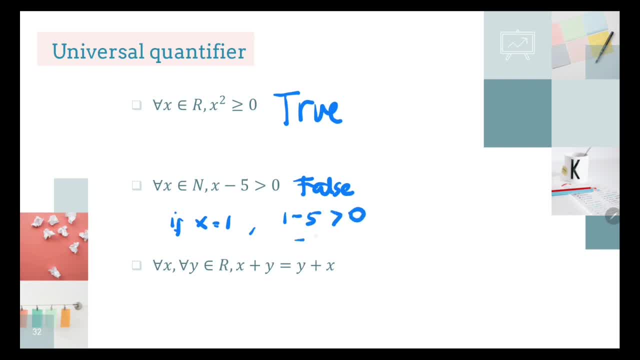 okay, so that would give me one minus five greater than zero, five greater than zero, five greater than zero, and that is negative. four greater than, and that is negative. four greater than, and that is negative. four greater than zero, zero, zero, which is a false statement. which is a false statement. 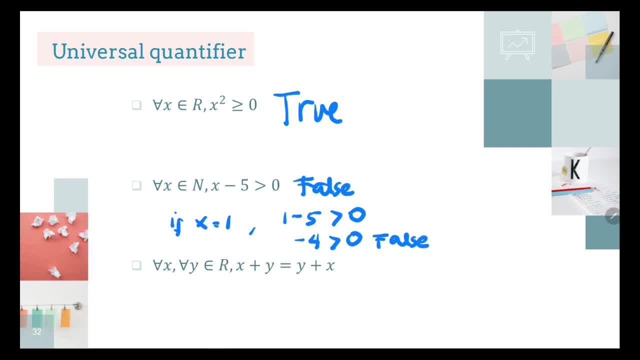 which is a false statement. okay, so that would mean the whole. okay, so that would mean the whole. okay, so that would mean the whole statement is statement, is statement is false, false, false, false, false, false. on the third one is on. the third one is on. the third one is true. 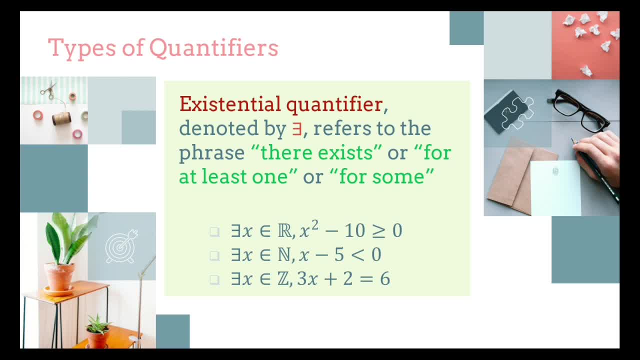 next we have the existential quantifier. next we have the existential quantifier. next we have the existential quantifier, denoted by, denoted by, denoted by. this symbol refers to the phrase there. this symbol refers to the phrase there. this symbol refers to the phrase there exists. 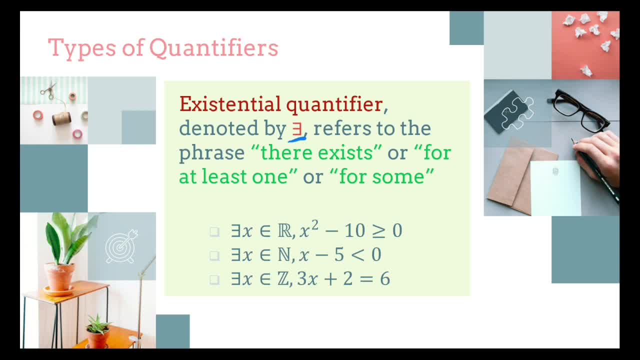 exists. exists or for at least one or for a sum, or for at least one or for a sum, or for at least one or for a sum. for example, there exists x. for example, there exists x. for example, there exists x. element of real number. element of real number. 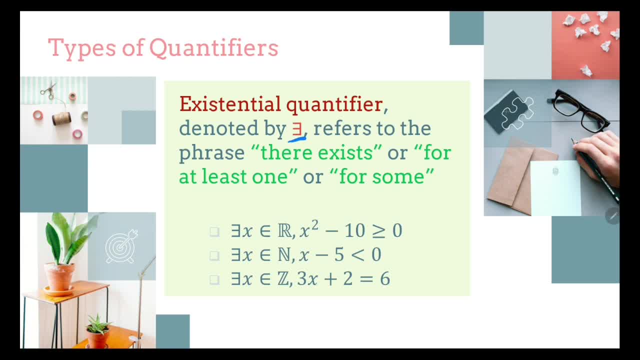 element of real number, such that x squared minus 10, greater than such that x squared minus 10. greater than such that x squared minus 10, greater than, or equal to zero, or equal to zero, or equal to zero. there exists an x element of natural. there exists an x element of natural. 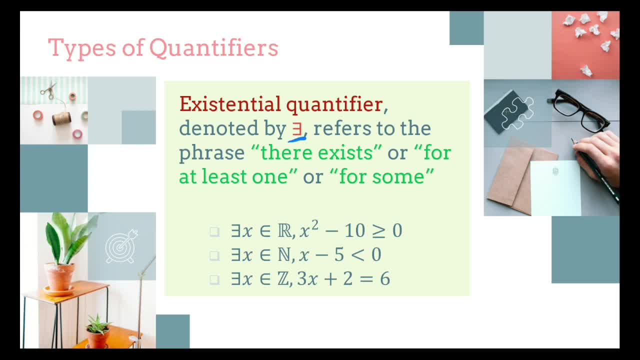 there exists an x element of natural numbers: x minus five numbers. x minus five numbers. x minus five is less than zero, is less than zero, is less than zero. and the third one. there exists an x and the third one. there exists an x and the third one. there exists an x element of integers. 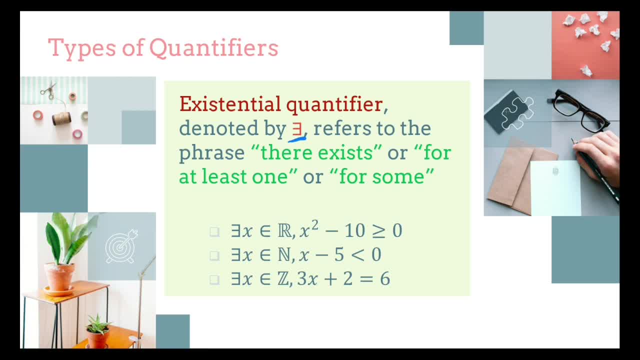 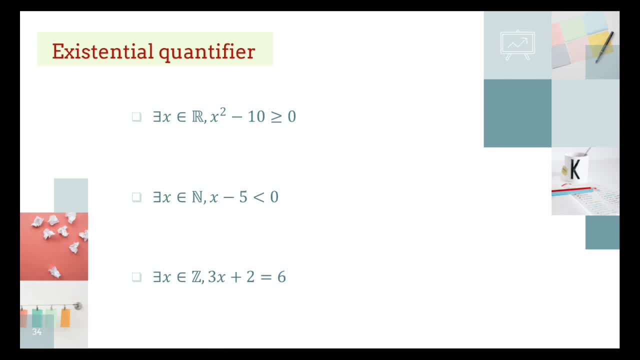 element of integers. element of integers such that three x plus two is equal to, such that three x plus two is equal to, such that three x plus two is equal to six. let's try to find, let's try to find, let's try to find their truth value: there exists an x. 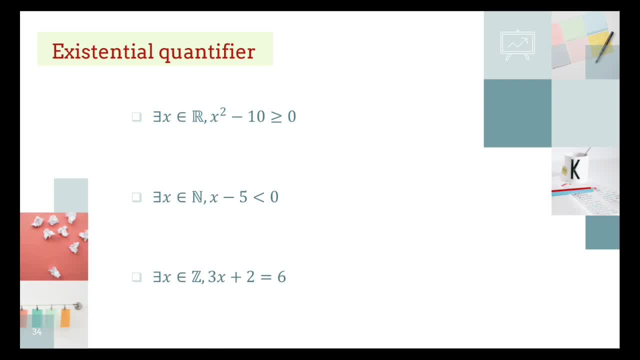 their truth value. there exists an x, their truth value. there exists an x. element of real numbers. element of real numbers. element of real numbers, such that x squared minus 10 is greater, such that x squared minus 10 is greater, such that x squared minus 10 is greater than or equal to zero. if we can find at: 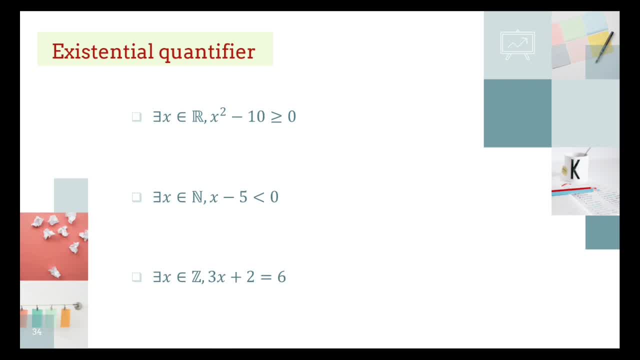 than or equal to zero, if we can find at than or equal to zero, if we can find at least one, least one, least one, one value of x. let's say, for example, one value of x. let's say, for example, one value of x. let's say, for example, if x is equal to four. 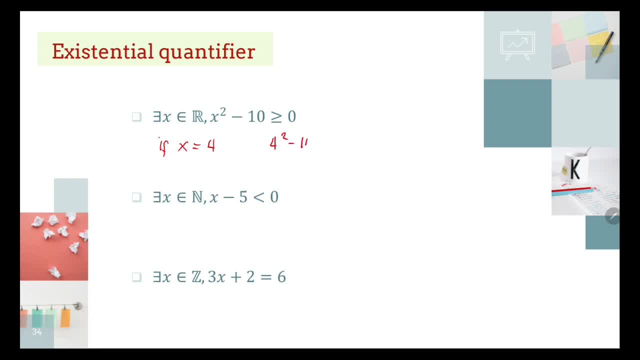 if x is equal to four, if x is equal to four, so that would give me four squared minus. so that would give me four squared minus. so that would give me four squared minus 10. 10, 10 greater than equal to zero. so 16 greater than equal to zero, that is six. 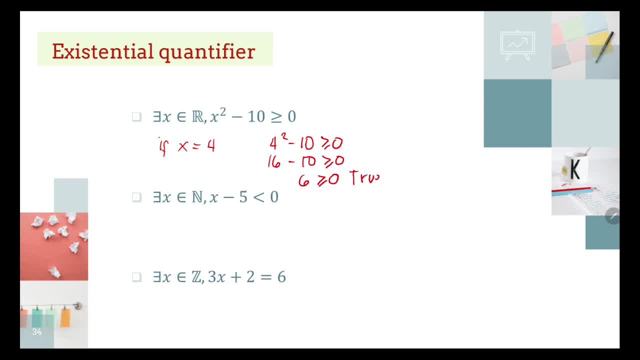 greater than equal to zero. so this is greater than equal to zero. so this is greater than equal to zero. so this is true, true, true. so i was able to find one at least one. so i was able to find one, at least one. so i was able to find one, at least one. so that would mean the whole statement. 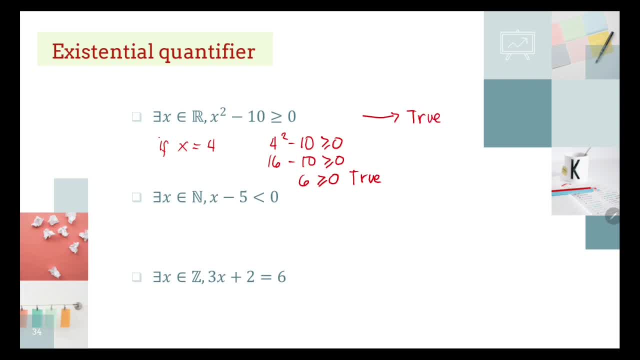 so that would mean the whole statement. so that would mean the whole statement is true, is true, is true. next, there exists an element. next, there exists an element. next, there exists an element of natural numbers. so one, two, three of natural numbers. so one, two, three of natural numbers. so one, two, three, four, five, six, seven, eight, nine, ten. 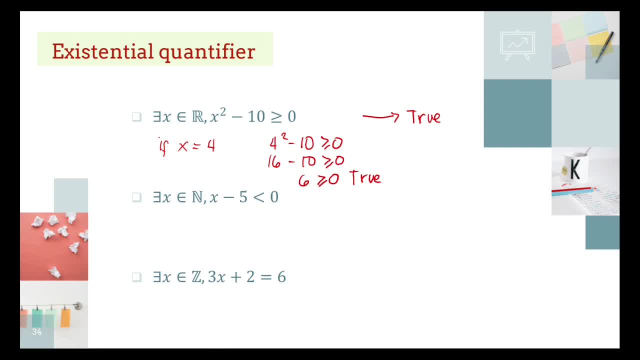 four, five, six, seven, eight, nine, ten. four, five, six, seven, eight, nine, ten, that would give x minus, that would give x minus, that would give x minus five less than zero, five less than zero, five less than zero. so let's say so, let's say so, let's say: if your x is also four, 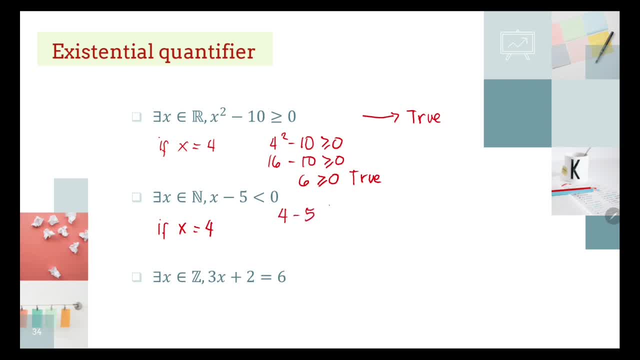 if your x is also four, if your x is also four. so that would be so. that would be so. that would be four minus five less than zero. that's four minus five less than zero. that's four minus five less than zero. that's negative one, negative one. 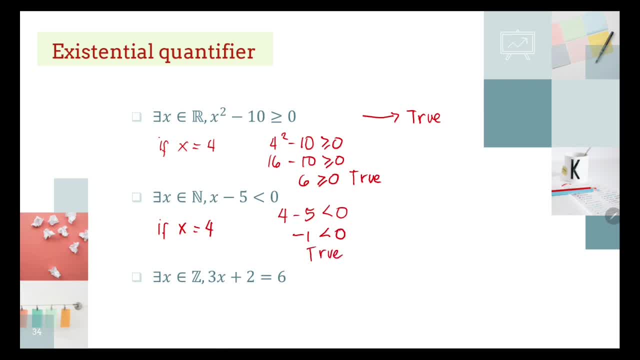 negative one, zero, which is true. then again, i was able- zero, which is true. then again, i was able- zero, which is true. then again, i was able to find, to find, to find one value element of natural numbers, one value element of natural numbers, one value element of natural numbers that would make the statement true. 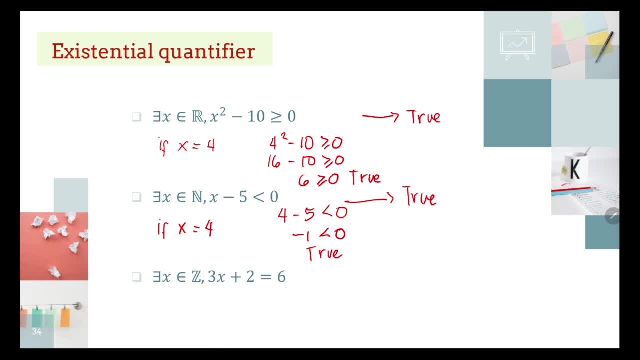 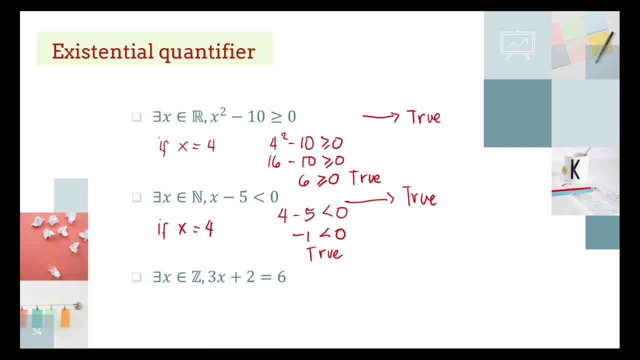 there exists, though, an integer. there exists, though, an integer that 3x plus 2 is equal to 6, that 3x plus 2 is equal to 6, that 3x plus 2 is equal to 6. okay, so, if we try to find, 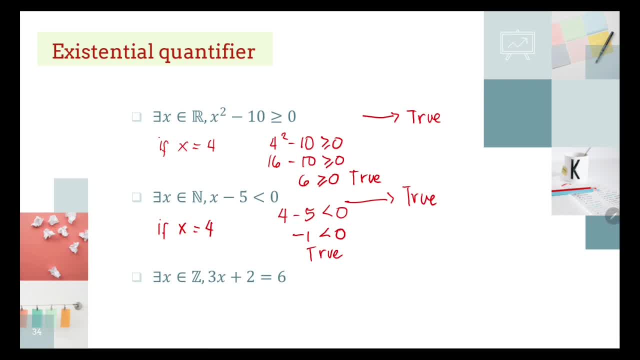 okay, so if we try to find, okay, so if we try to find that value that would make the statement that value that would make the statement, that value, that would make the statement true, true, true, i will try to solve this equation. i will try to solve this equation.